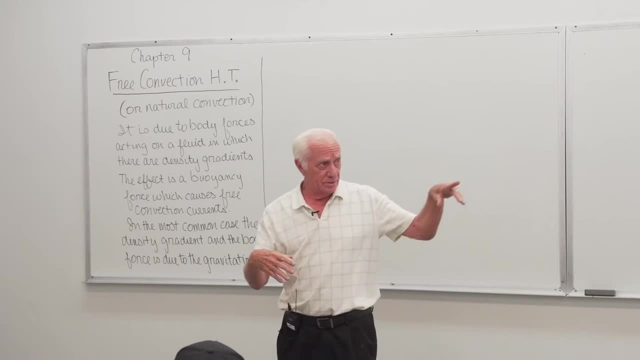 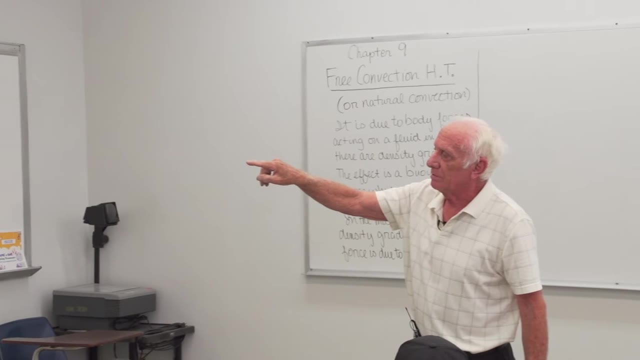 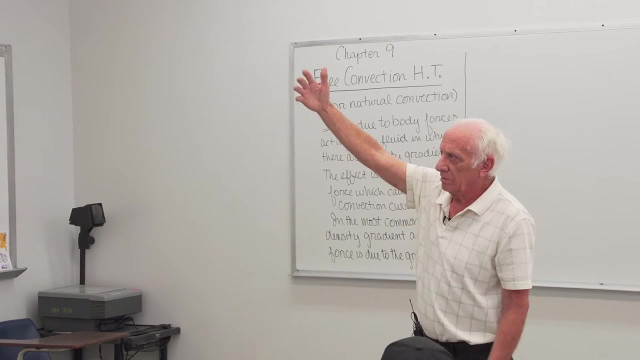 If this room is warm because of that outside wall being heated, the hall side wall is probably cooler because the hall is a cooler place. So the hall side wall is cooler. The air on that wall gets more dense because it's colder and it drops down to the floor. 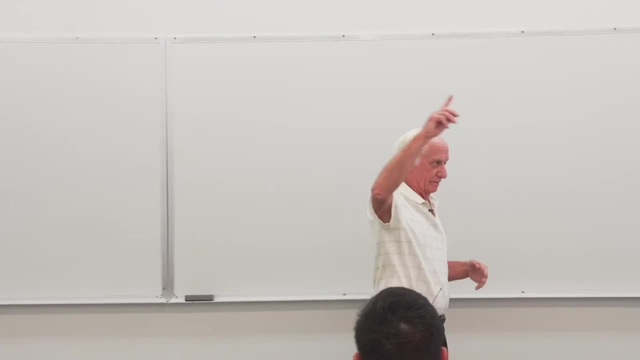 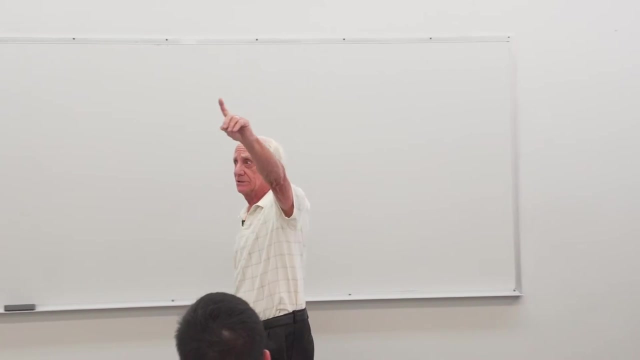 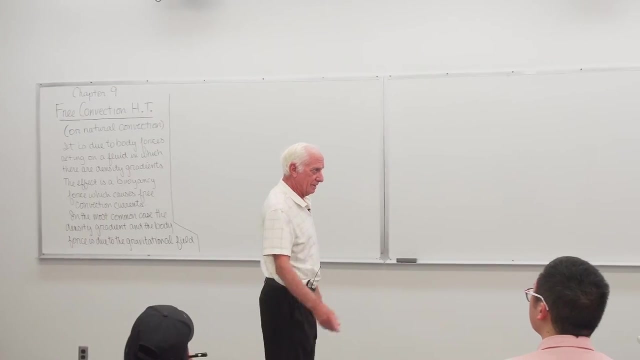 So you can get a cycle of air in here. Warm air rises up across the ceiling to the hall side wall. where it's colder, It drops, It goes across the floor So you can get motion. that way It's natural or free. 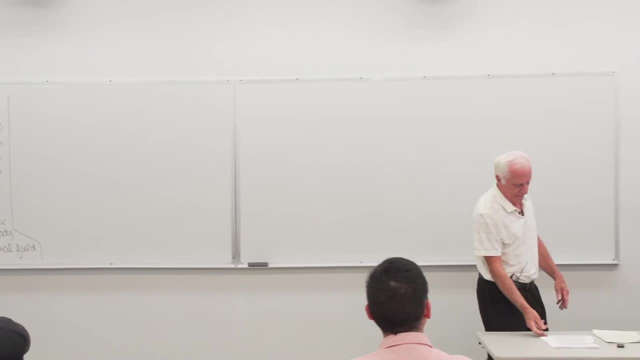 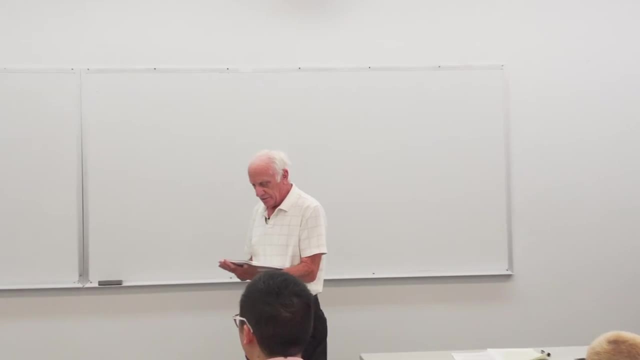 Natural or free. So the textbook. in the introduction of Chapter 9, there are some interesting comments, So I just want to go over that with you. I photocopied that first page in Chapter 9, and I'll read it with you. 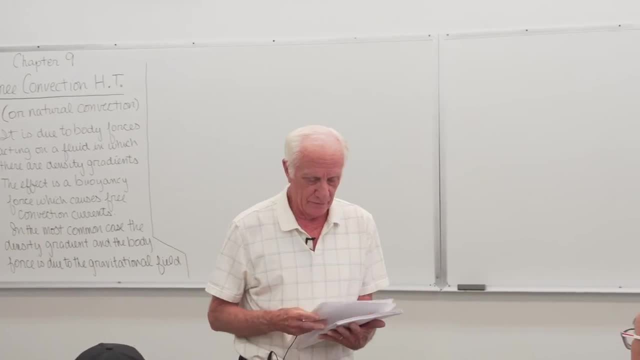 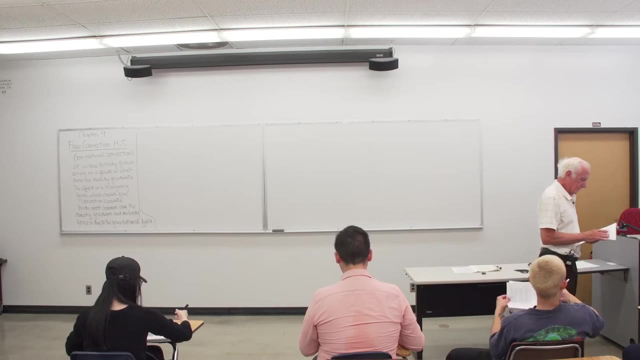 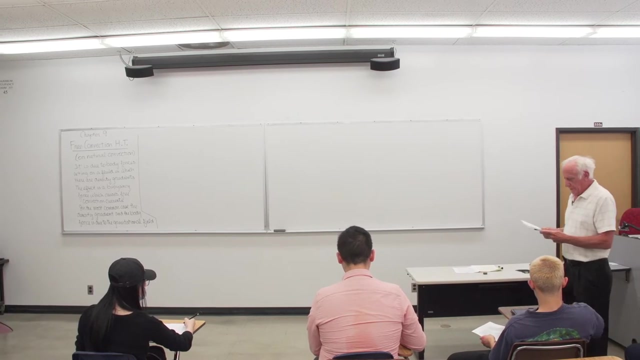 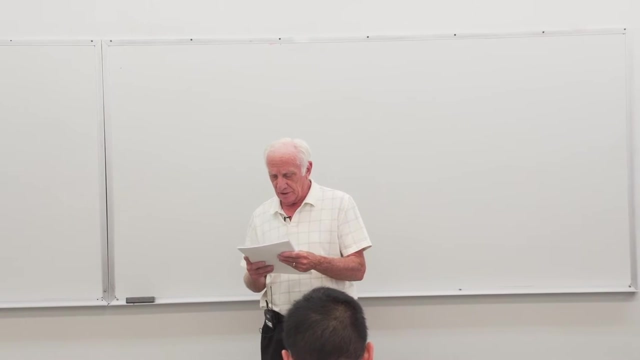 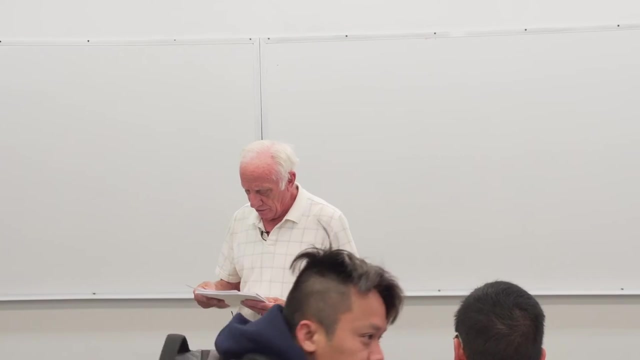 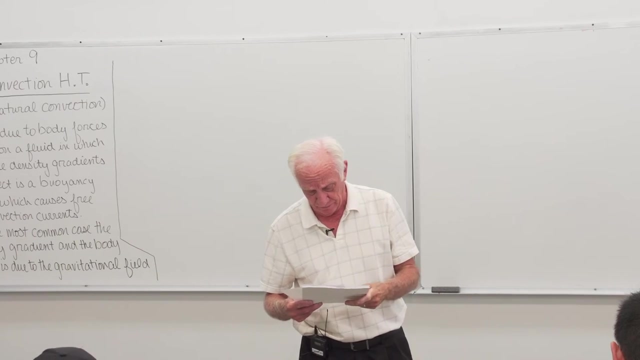 So where the arrows are there, it says. Since free convection flow velocities are generally much smaller than those associated with forced convection, the corresponding convection heat transfer and the heat transfer rate are also smaller. It's perhaps tempting to therefore attach less significance to free convection processes. 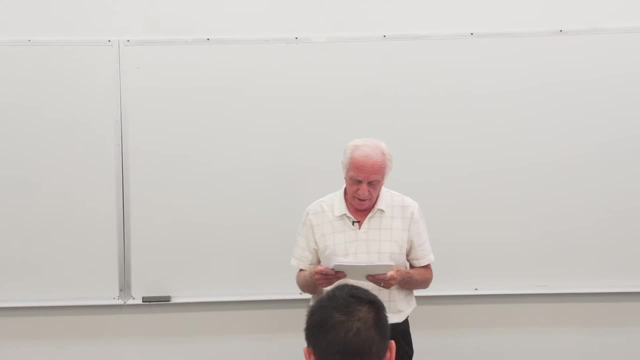 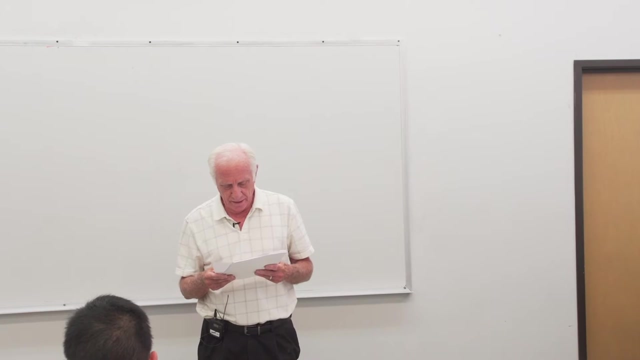 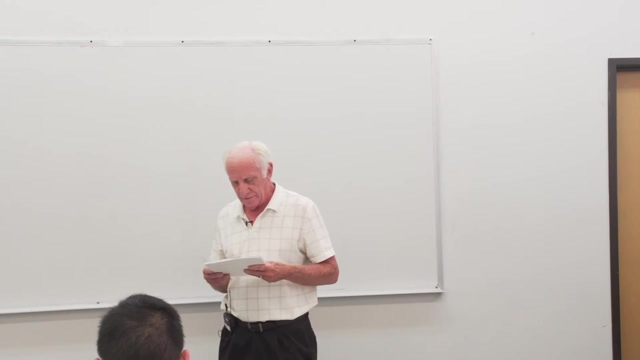 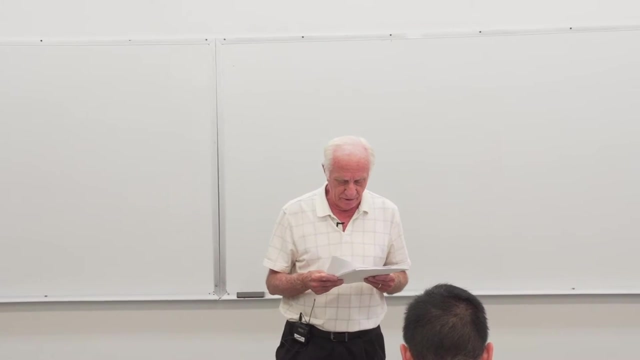 This temptation should be resisted. In many systems involving multimode heat transfer, that means conduction-convection. radiation free convection provides the largest resistance to heat transfer and therefore plays an important role in the design and performance of the system. Moreover, when it is desirable to minimize heat transfer rates or to minimize operating costs, 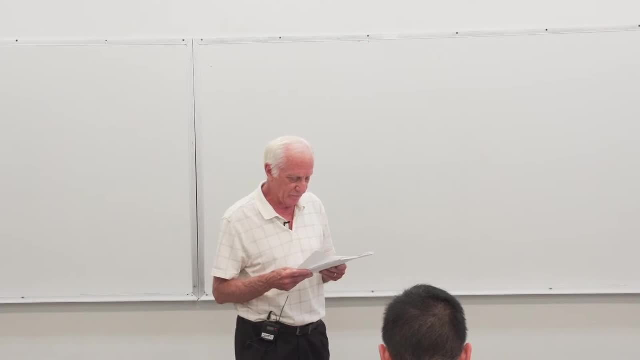 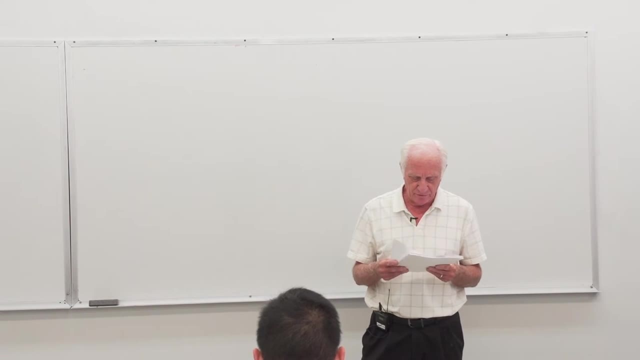 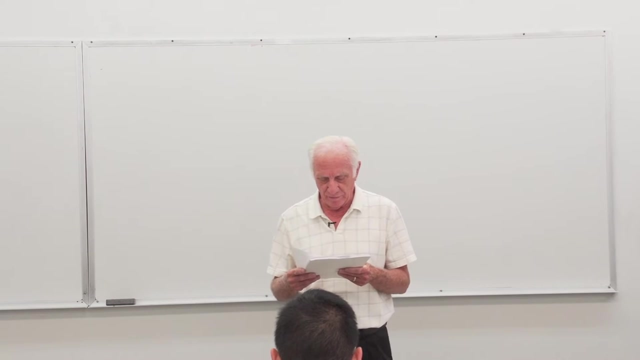 free convection is often preferred to forced convection. There are, of course, many applications. Free convection strongly influences the operating temperatures of power generating and electronic devices. It plays a major role in a vast array of thermal manufacturing applications. Free convection is important in establishing temperature distribution within buildings. 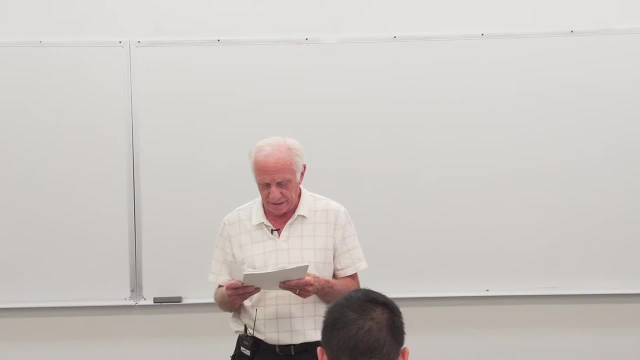 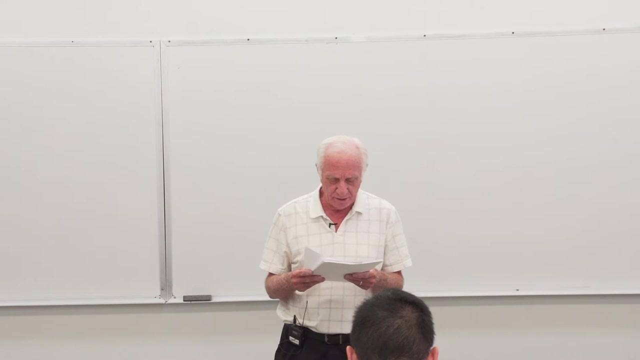 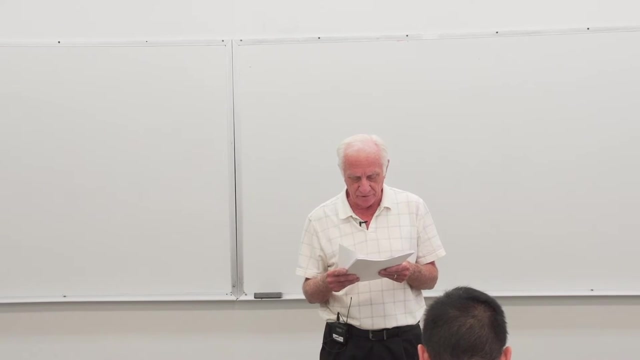 and in determining heat losses and heat loads for heating, ventilating and air conditioning systems. Free convection distributes the poisonous products of combustion during fire and is relevant to the environmental sciences where it drives oceanic and atmospheric motions. So yes, it plays important roles in our engineering world. 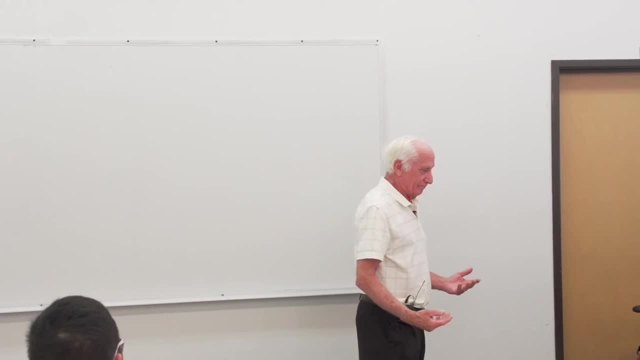 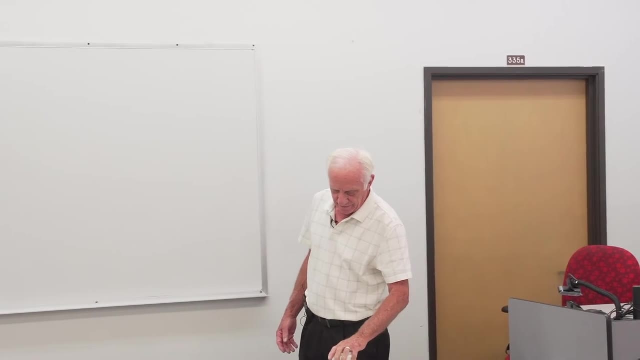 I mean, even if I, I mean, even if I, I mean, even if I, I want to keep my coffee heated until the end of my next lecture, which I'd like to have, but it's not going to work. 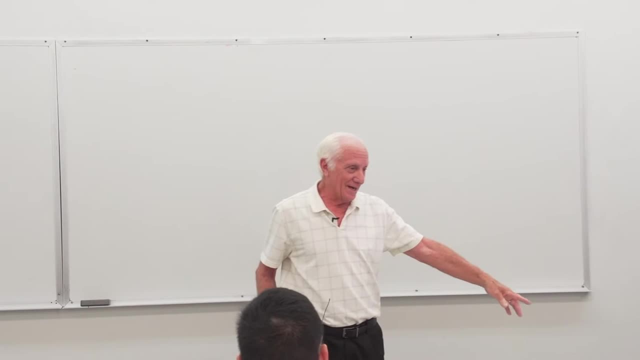 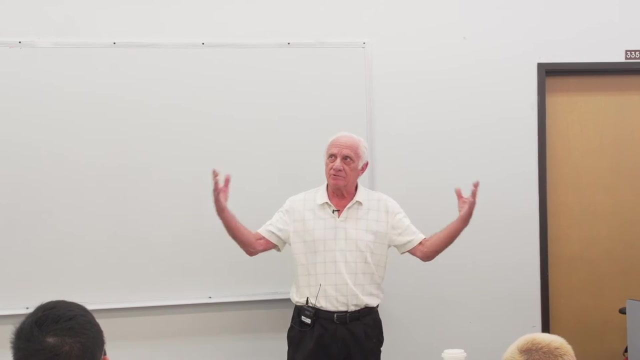 I don't want to put a floor fan here and blow over that, because I know what's going to happen. It's going to cool faster. So I turned the floor fan off and now this coffee's in this room where the air is not moving hardly at all. 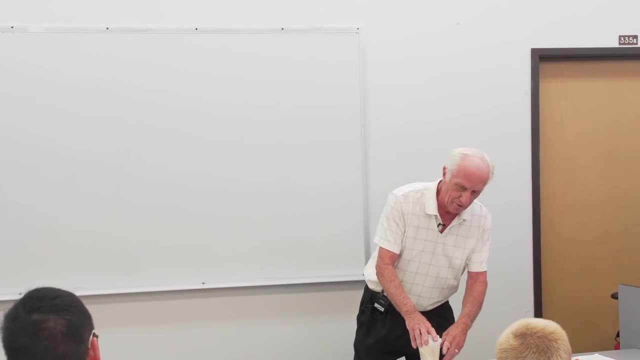 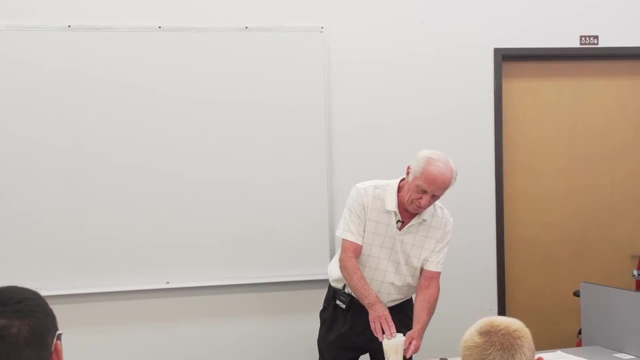 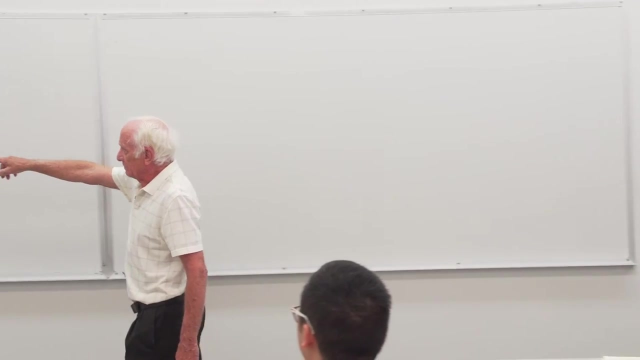 But the coffee right here is hot, The surface is hot. Guess what? I get a boundary layer built up here on the outside, a boundary layer caused by what Caused by these, Caused by density gradients and a buoyancy force pushes the air up. 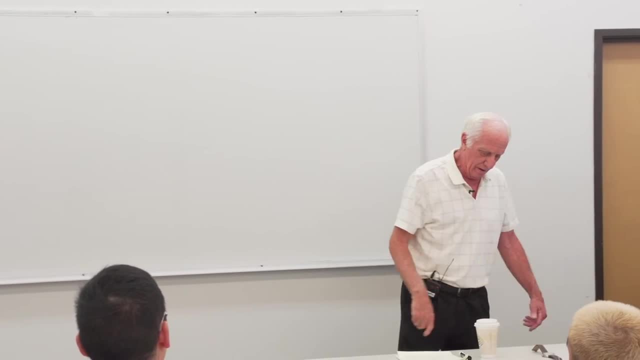 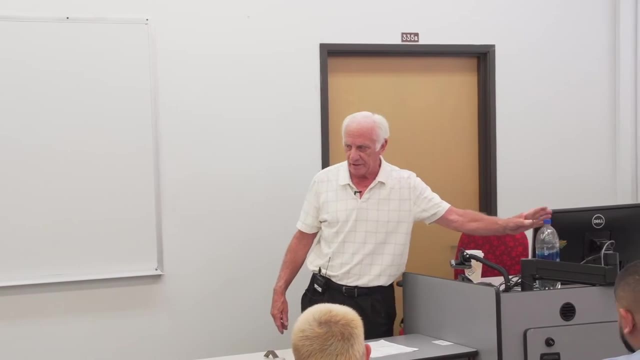 and creates a boundary layer over the perimeter of the cup. So, yeah, I want free convection, I don't want forced convection. Same thing with cool: You're carrying cold fluids around. Yeah, yeah, you want to keep them away. 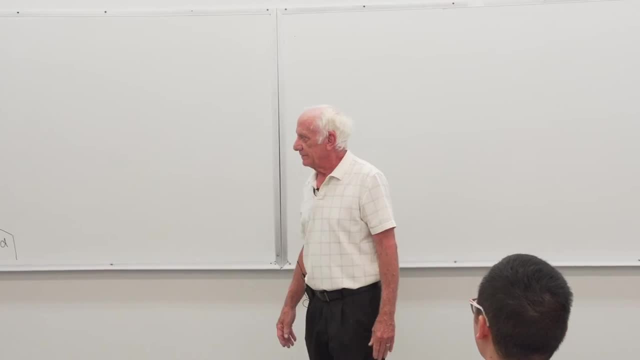 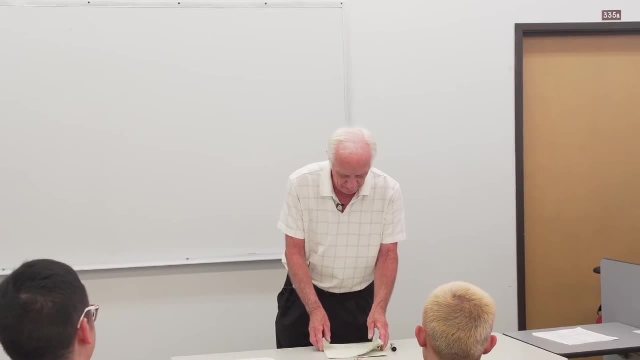 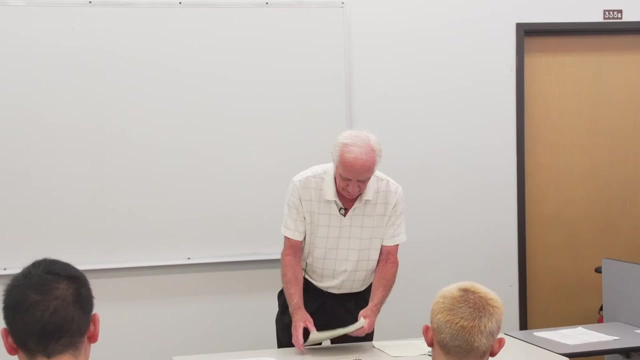 from hot air blowing over the cool drink. So it does appear a lot in our study of convection heat transfer And we're going to go back and take a look and contrast Chapter 9 to Chapter 7 and 8. So let's go back. 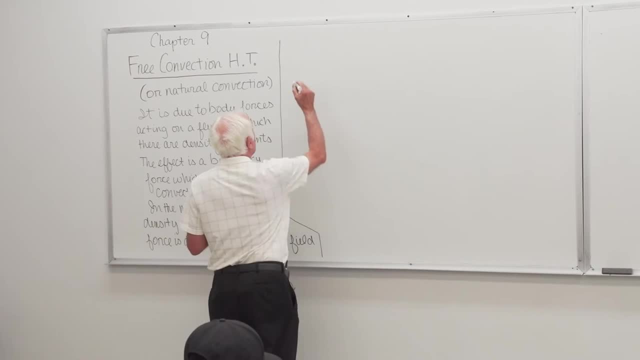 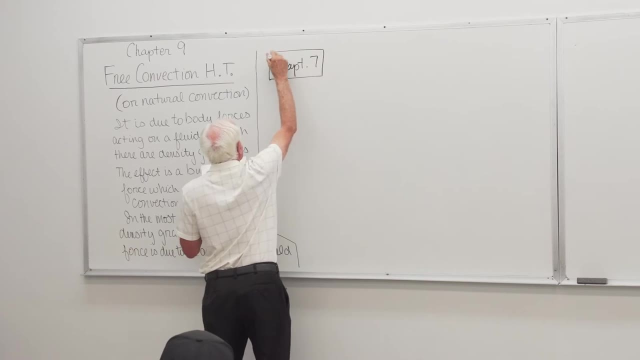 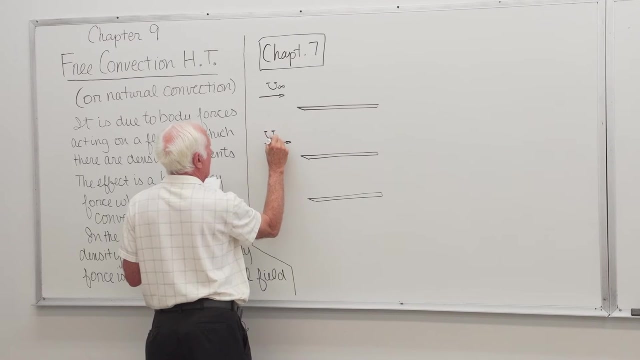 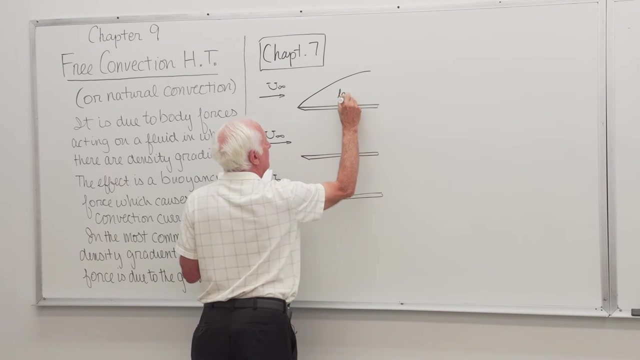 And look at Chapter 7.. Okay, so we have. I'll just summarize what we did in Chapter 7. here We could either have all-laminar boundary layer or maybe all-turbulent boundary layer, or we could have a mixed-flow boundary layer. 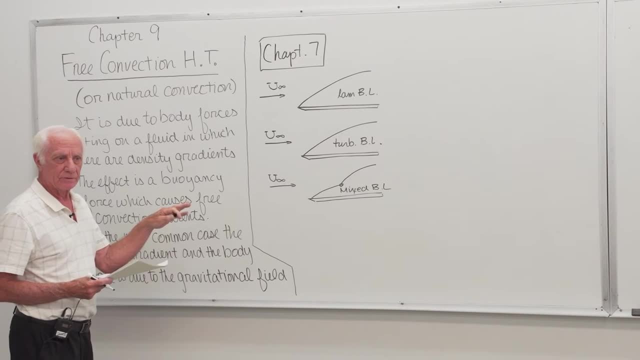 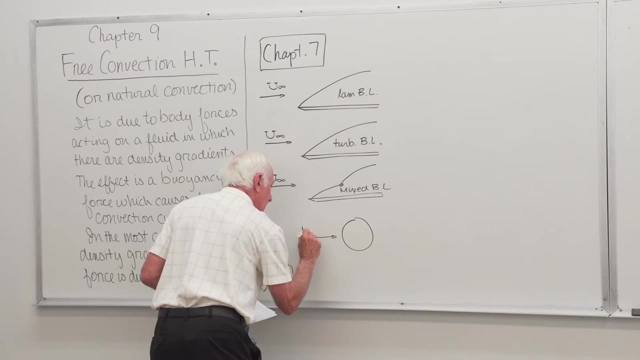 External flow, Flow over external surfaces, Or also Chapter 7, we can have flow around a circular cylinder. We could have a laminar boundary layer, a mixed boundary layer and a wake region. Diameter- Diameter: Diameter was D. 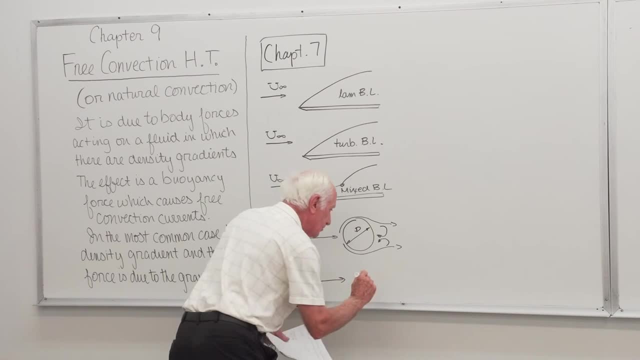 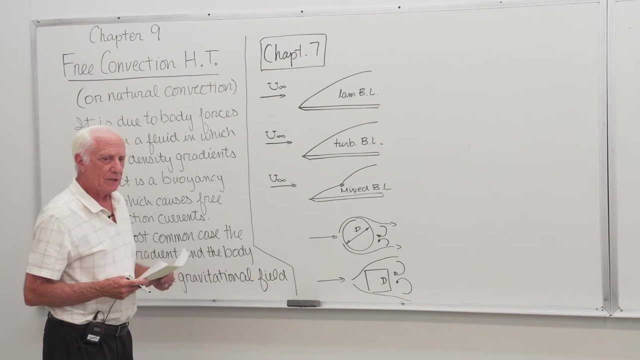 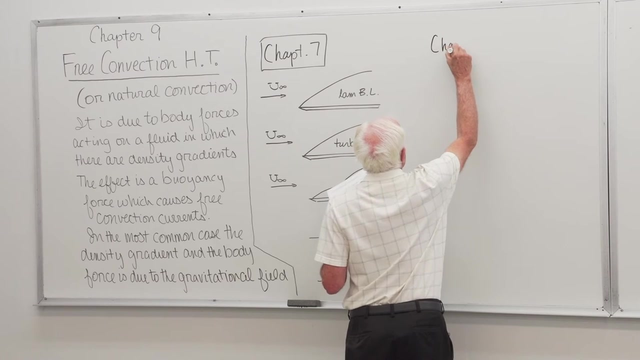 And we can also have- we looked at other geometries- Maybe a square tube like this, Each side dimension D. So that was Chapter 7, external flow. Now we do Chapter 8.. Chapter 8. Tube flow- Internal flow. 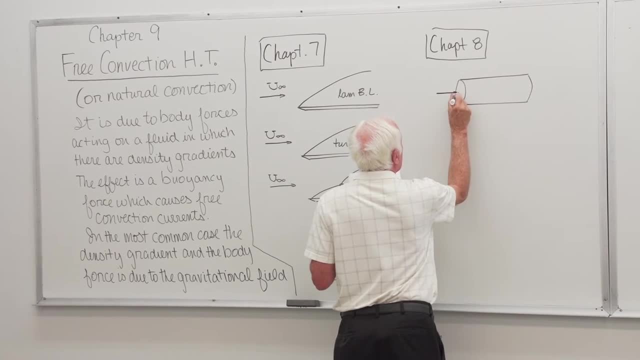 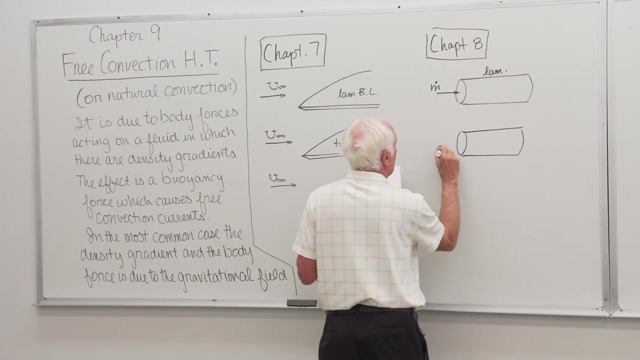 Convection heat transfer. Have a mass flow rate m dot, for instance. This can be laminar flow. Então, this is a mass flow rate. This is a mass flow rate. This can be turbulent flow. Let's put the velocity on here. 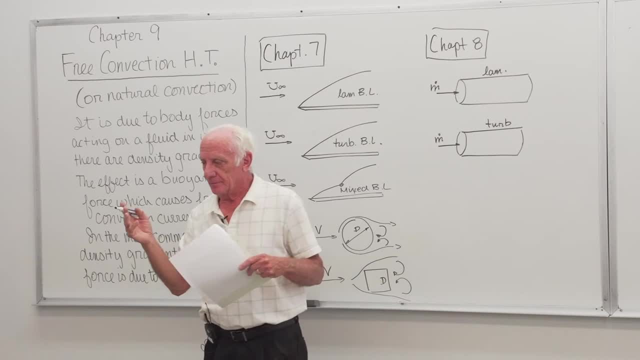 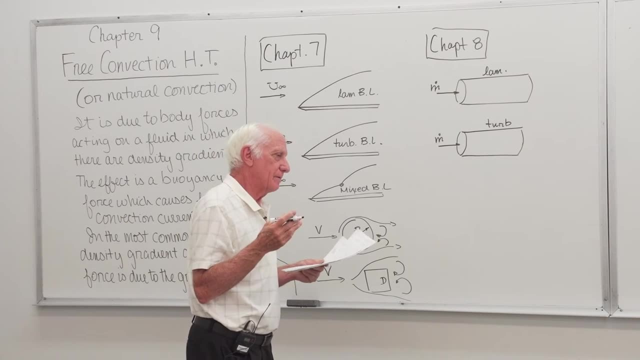 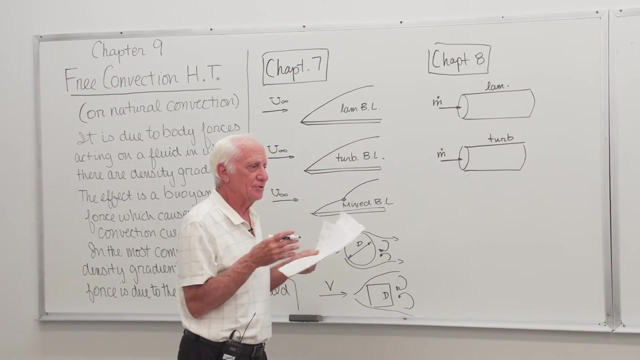 Laminar flow? is a constant surface temperature? Is a constant surface heat flux? Is it fully developed velocity? Is it fully developed temperature? Answer all those questions. it leads you to what? H? Turbulent flow. we only had one equation. 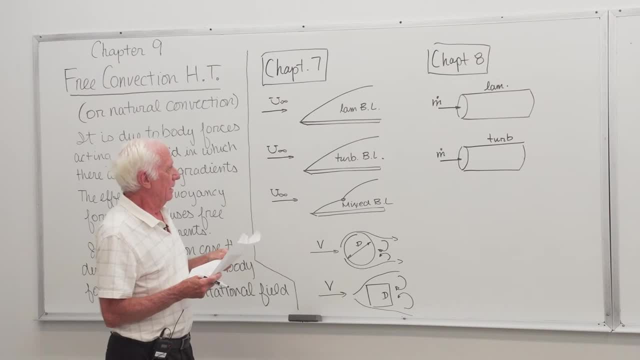 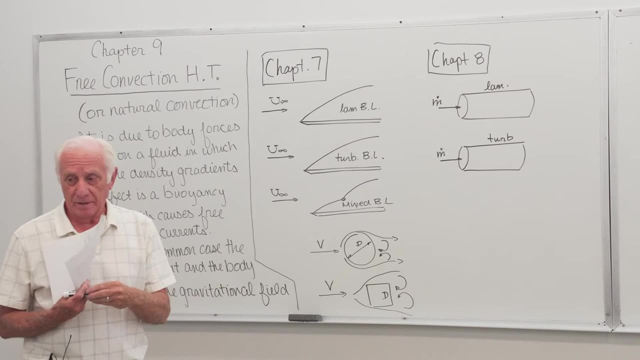 good for everything. What does it give you? H, Every one of these guys. the objective in Chapter 7 and 8, number 1, find H, Because once you find H, you can now find the heat transfer or other important things going on. 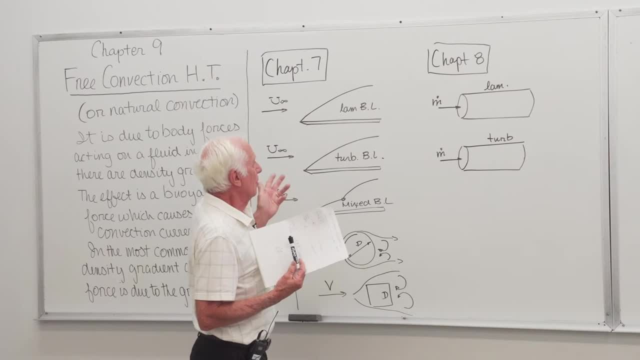 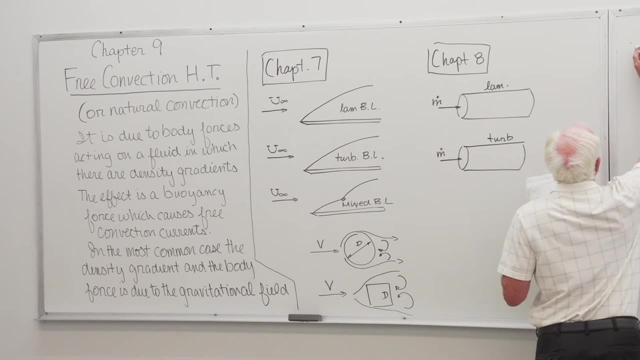 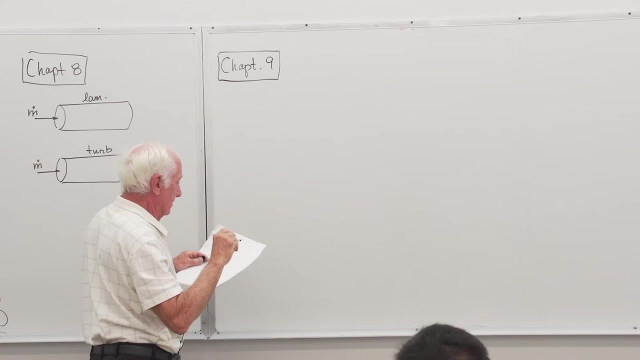 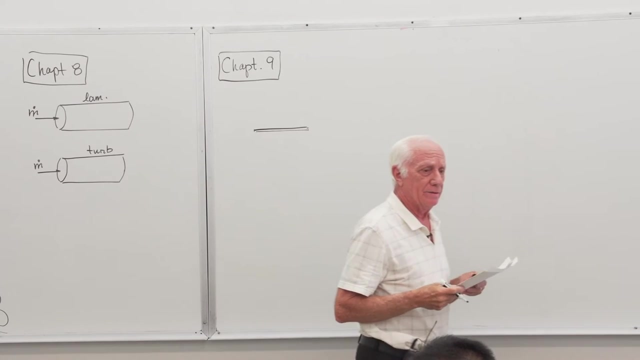 Typically we found heat transfer, So get H, find Q. So now we go to Chapter 9.. I'll give you different geometries. The first one: I'm going to have a heated horizontal plate, So it's like a hot plate in the kitchen. 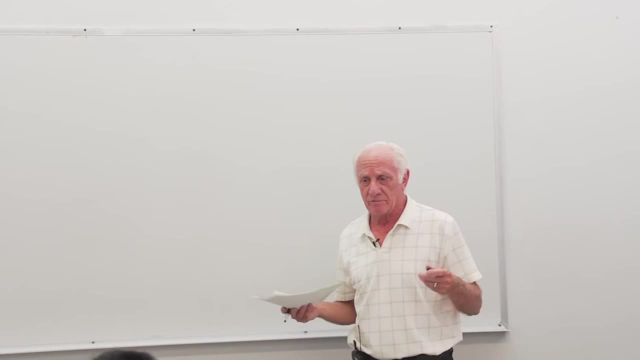 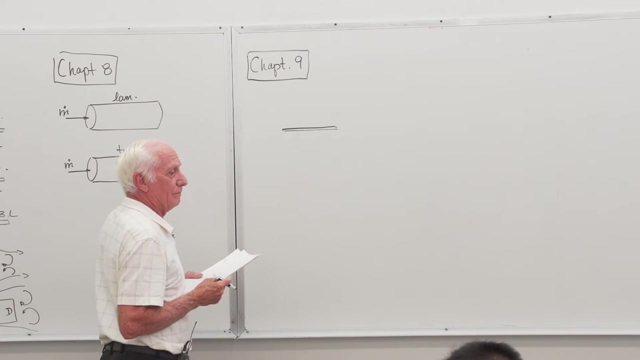 You plug in the wall the hot plate. it gets hot. you do whatever: Heat your coffee on it, heat a soup on it, whatever. But what's happening is: is there a fan in the kitchen blowing over it? No, 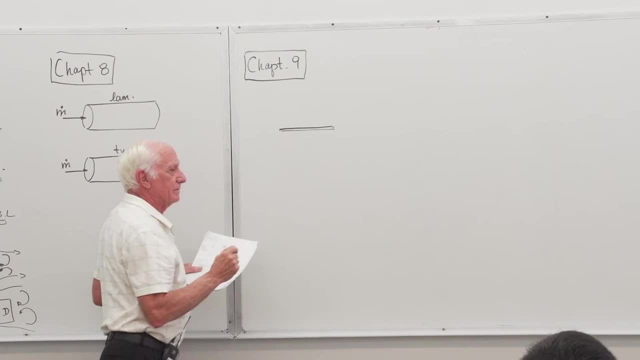 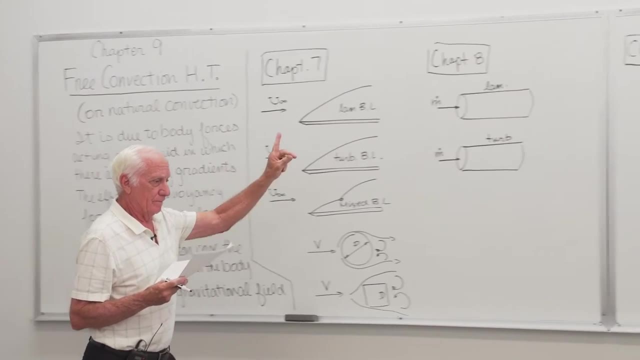 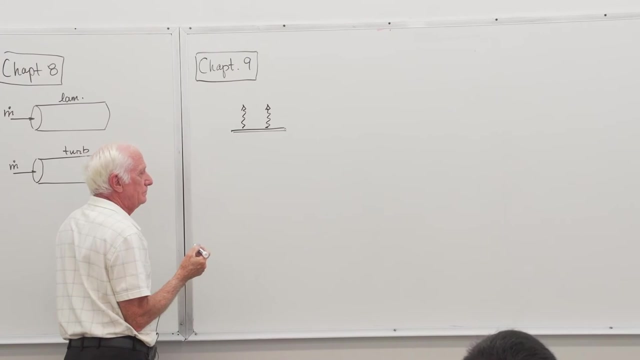 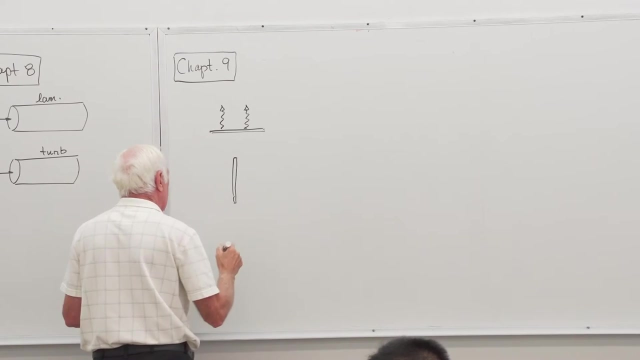 But the air close to the heated surface, its density goes down. There's a buoyancy force, The air wants to rise, So the heated air is rising off of the surface. Then you can turn this, so now it's a vertical surface and now you have heated. 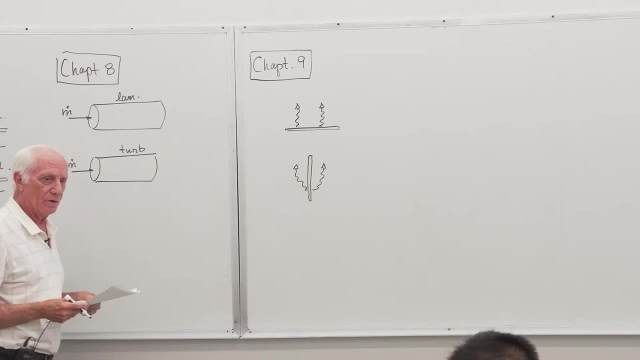 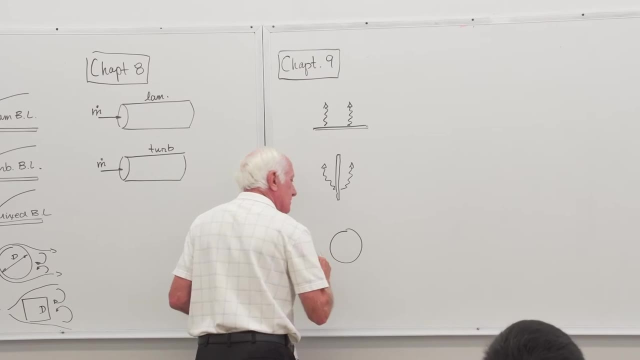 Let's say it's heated and of course the air again wants to rise because of buoyancy effects, density gradients. Then you could have, for instance, circular cylinders and again heated, and so the air is rising off of the heated circular cylinder. 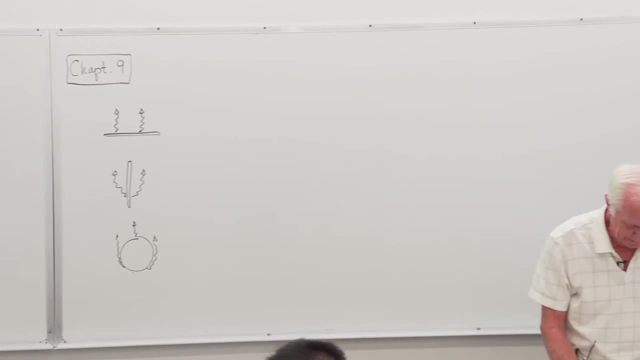 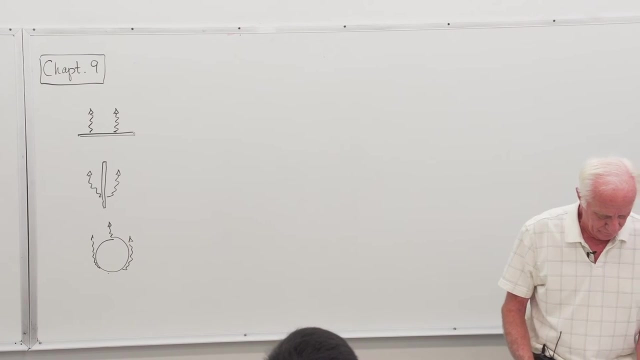 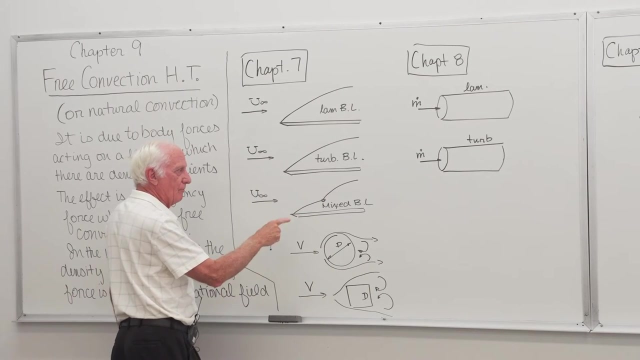 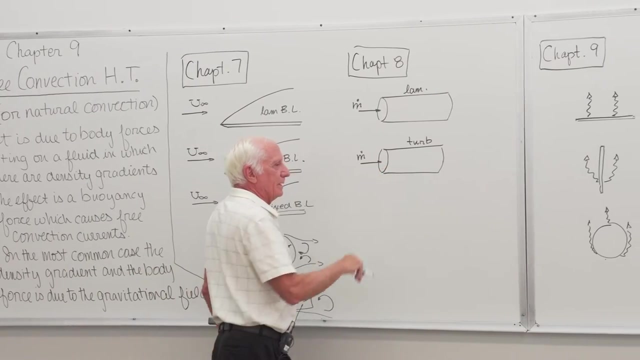 So that's what we're going to be looking at in Chapter 9,, which is different. Chapter 7, something is forcing the fluid over the external surface- A fan, for instance. Chapter 8, something is forcing the fluid through the tubes. 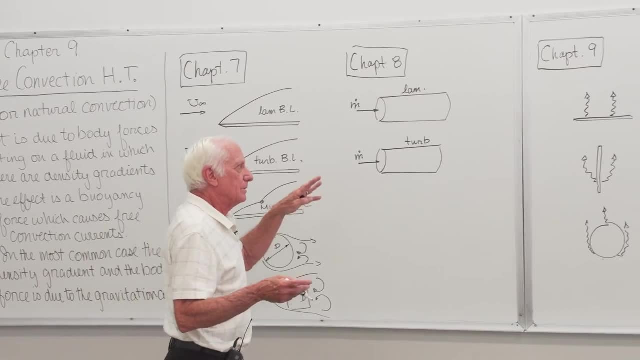 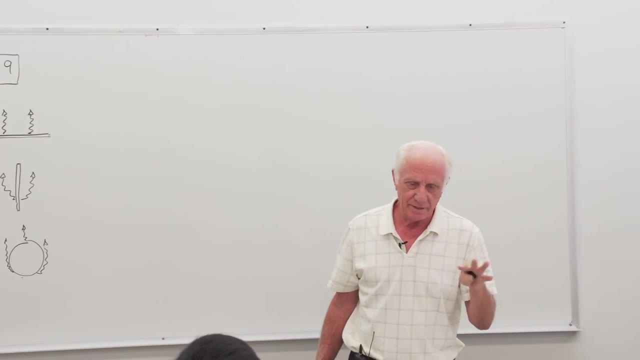 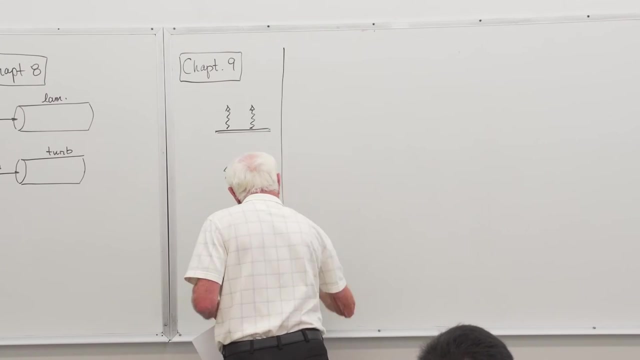 Maybe a pump. Chapter 9, there's no fans, there's no pumps. it's due to natural or free convection. Okay, So that's Chapter 9.. If you go back and look, just as a summary, Table 1.1, Chapter 1, Table 1.1.. 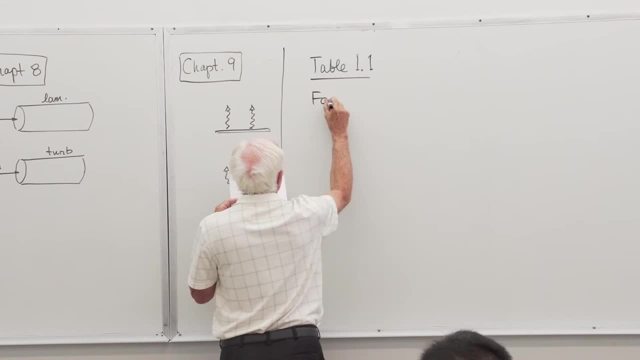 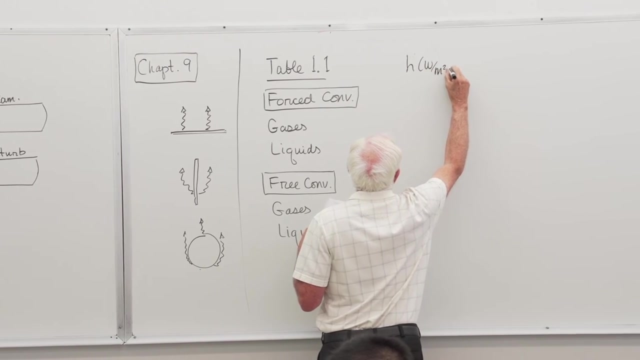 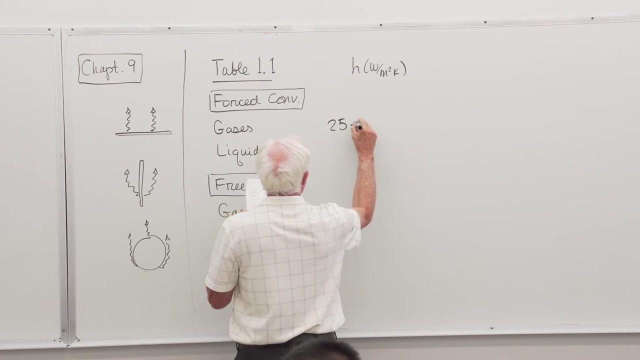 Forced convection gases and liquids. Free convection gases and liquids. He gives you a typical range of h-values: Gases: 25, to 250.. Liquids: 100 to 20,000.. Free convection gases: 2 to 25.. 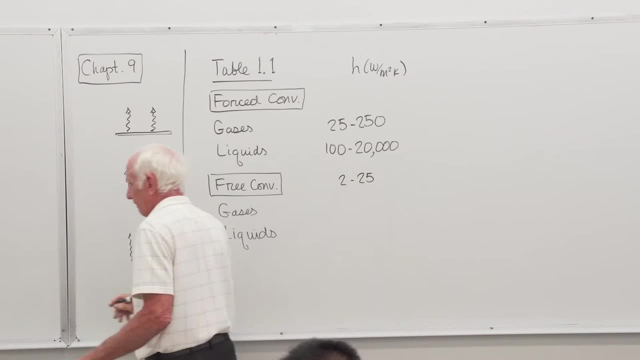 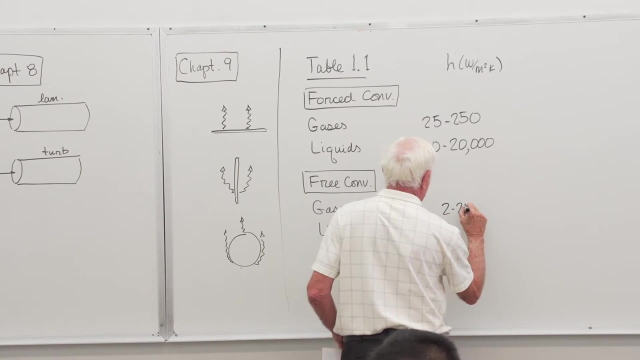 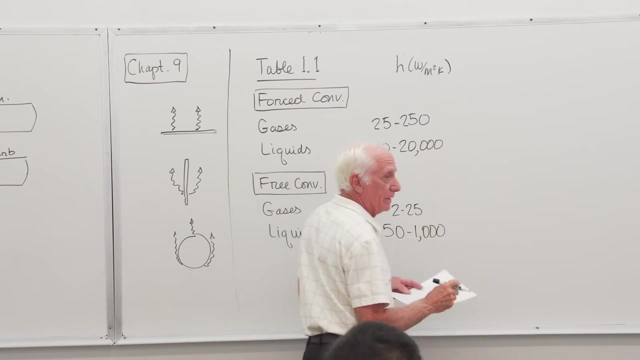 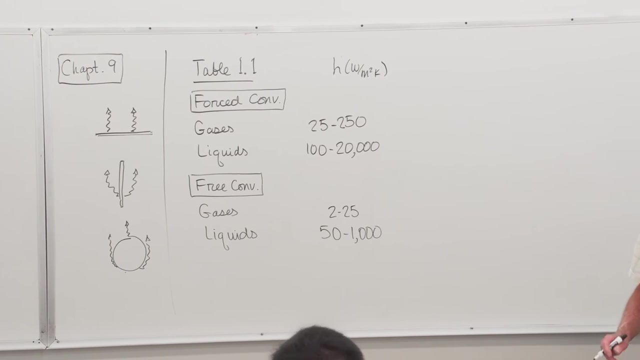 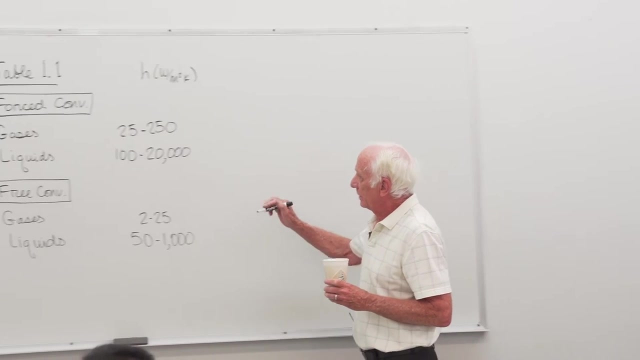 25.. Liquids: 50 to 1,000.. Oh yeah, there's a major difference in those guys. You can see major difference. 20 to 1,. 10 to 1, gases: high-value: 25, free convection gases. 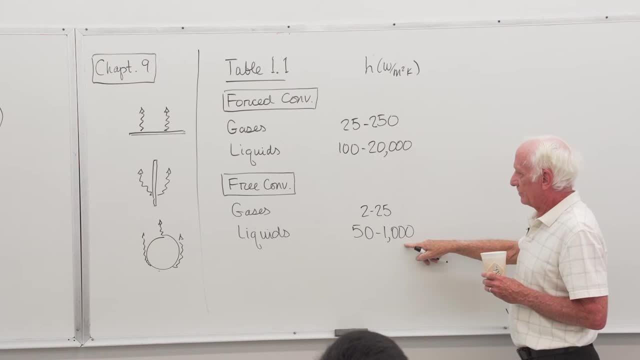 forced convection: 10 times higher. High-value for liquids: free convection: 1,000.. 20,000, 20 times higher, Two times higher, 12 and a half times higher. Yeah, Don't forget now the resistance. 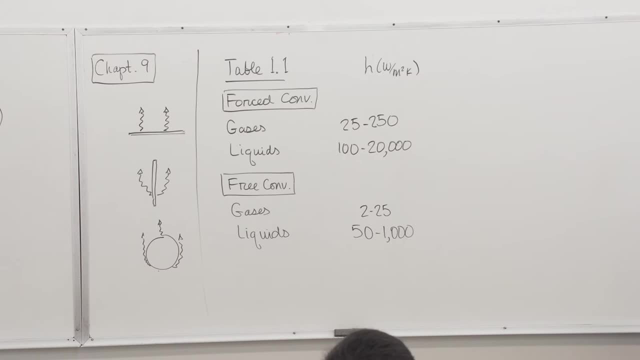 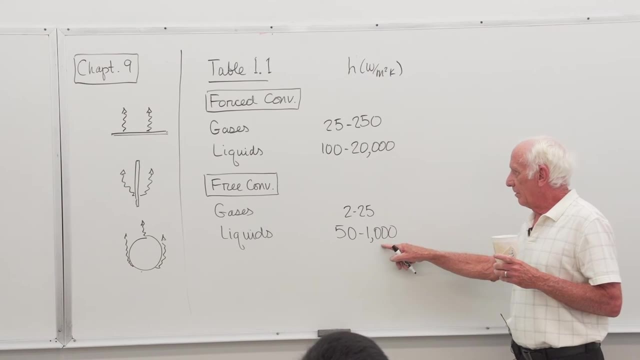 if you model it as a resistance convection, heat transfer, it's 1 over h-a, So the smaller h's have the bigger resistances. Big resistance, smaller resistance, Big resistance, smaller resistance, Free convection: 25, 250.. 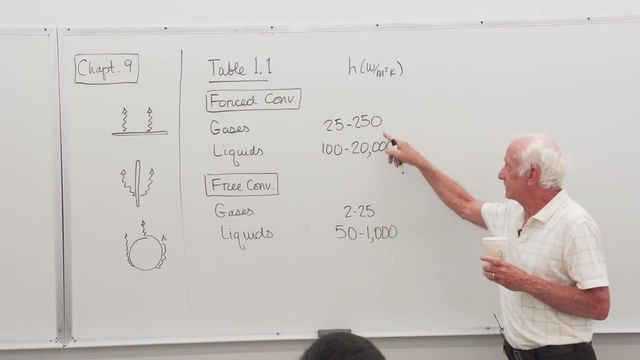 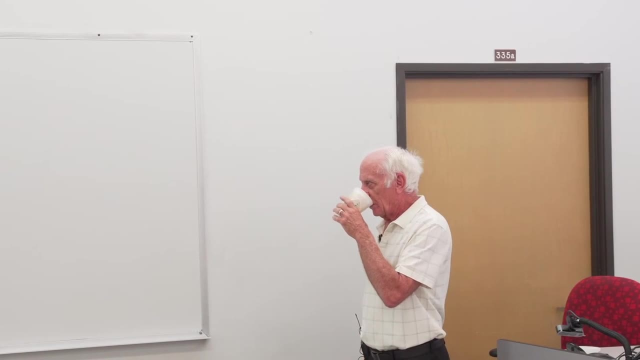 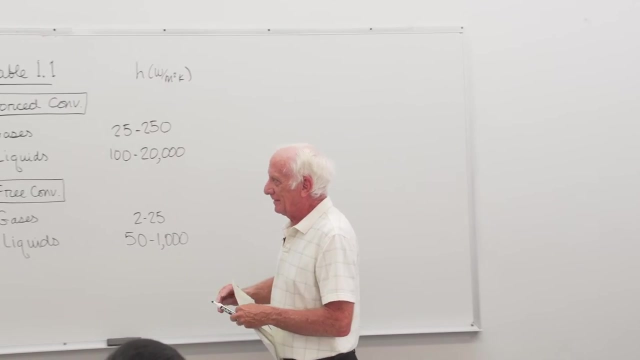 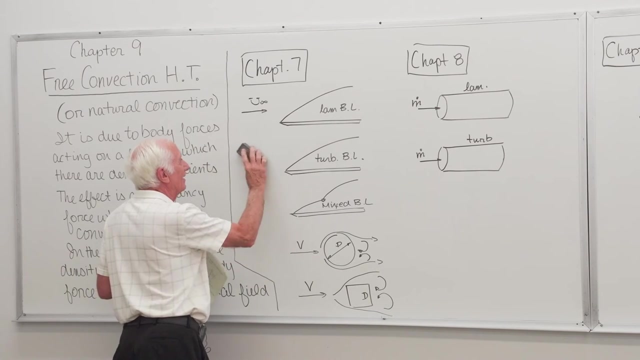 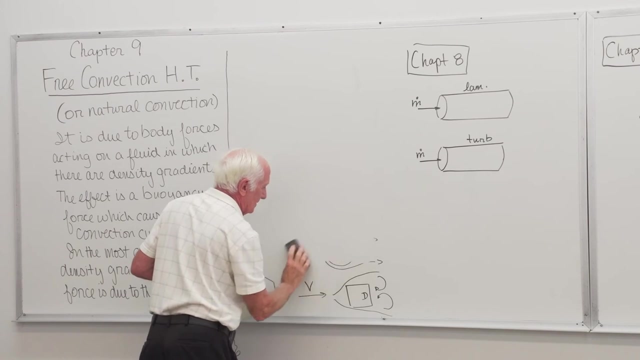 One over h. Big number, big resistance, Smaller resistance. So that's what we're looking at in Chapter 9.. This just gives you an idea of what's going on before we get to the real engineering part. So we're going to look at what's. 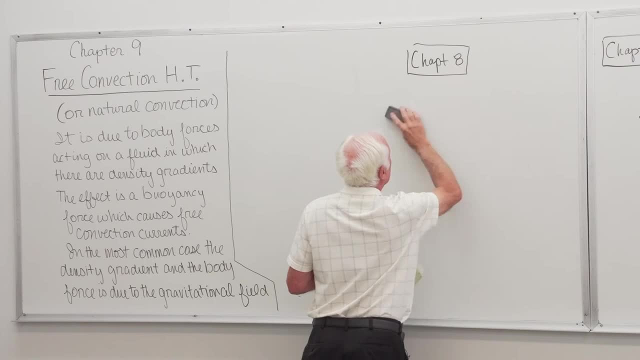 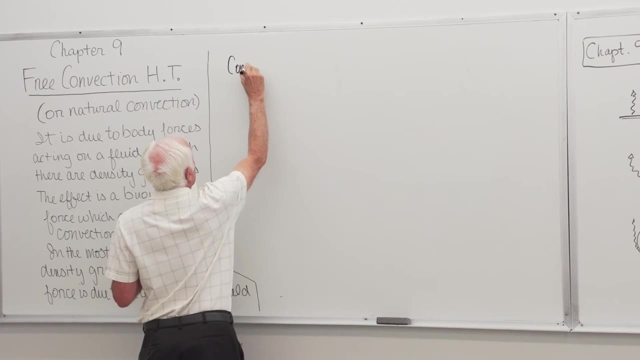 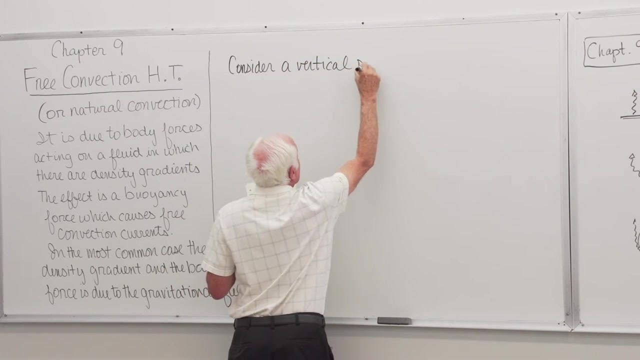 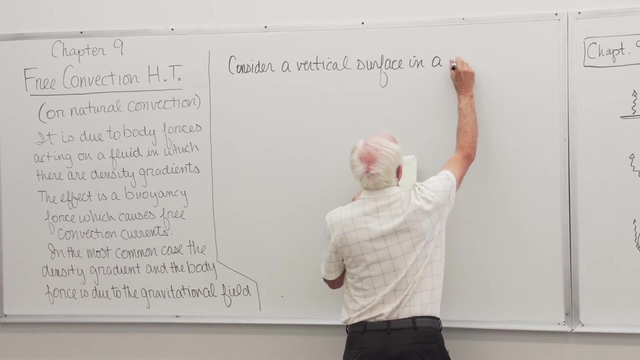 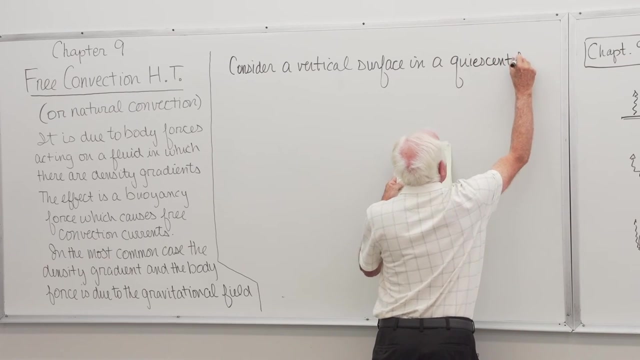 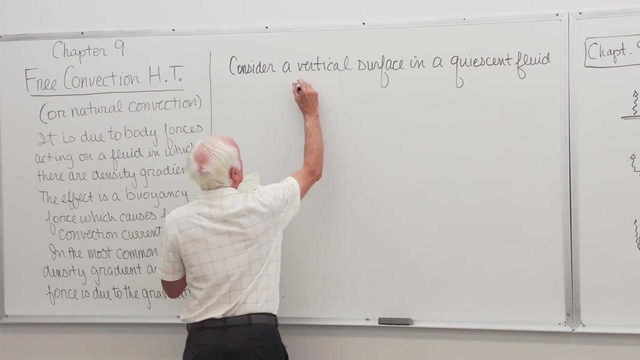 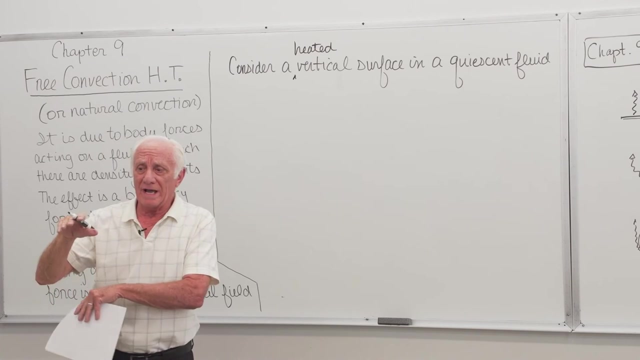 happening in free convection in more detail. So we're going to start out and we're going to consider a vertical surface in a quiescent fluid. We're going to consider it's heated, so consider it heated. Quiescent means still quiet, not moving. 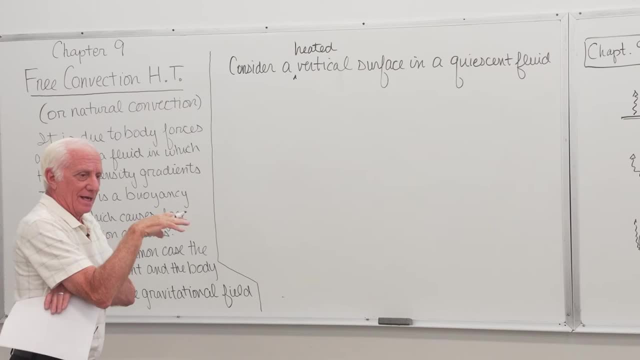 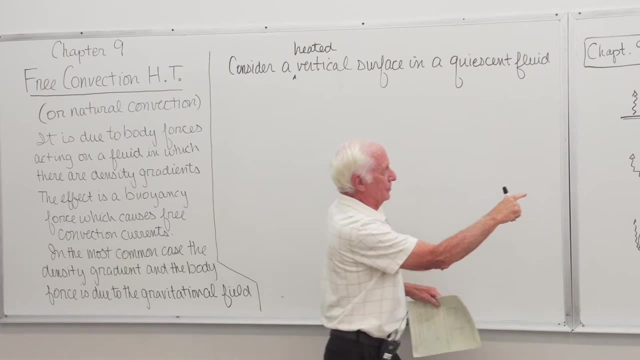 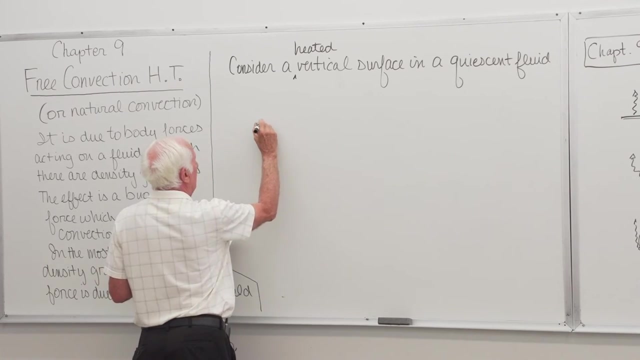 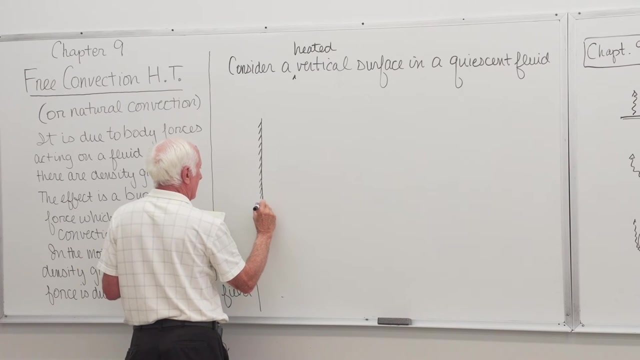 Quiescent means not moving. still Velocity is zero. So we'll look at the vertical plate first, because that's a simple geometry. There's a vertical plate, So I have this vertical plate. I'm going to measure y this way. 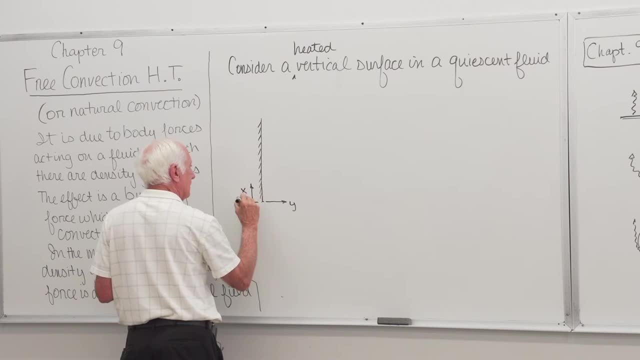 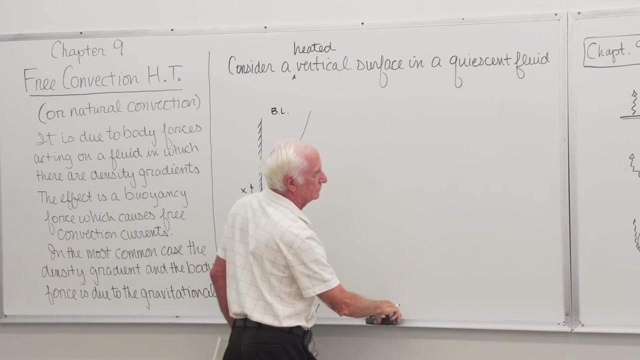 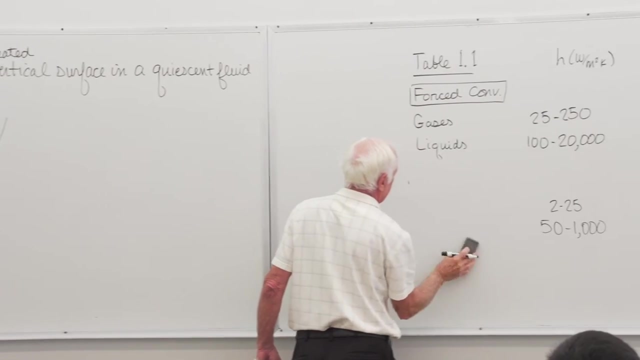 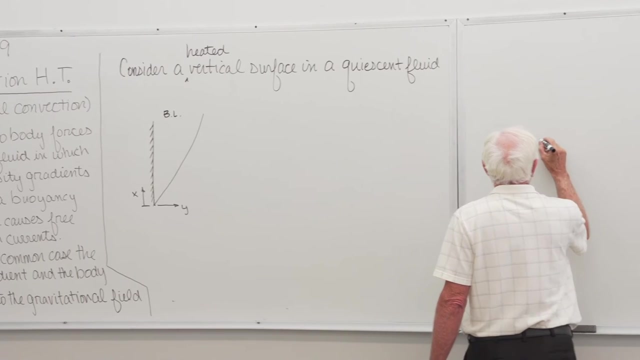 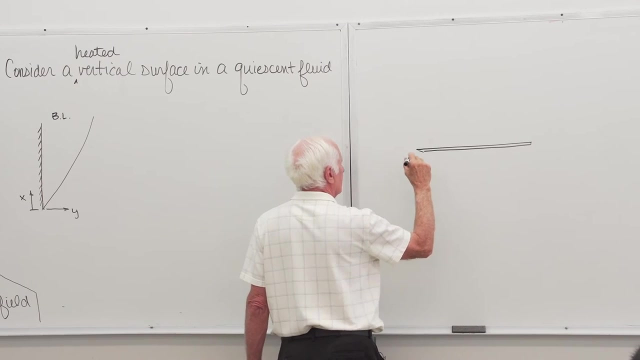 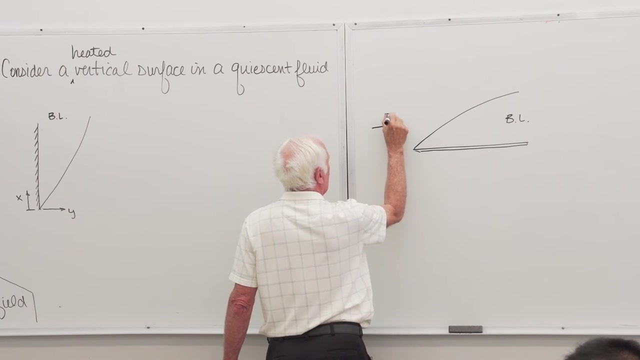 I'm going to measure x this way. The surface is heated, The fluid starts to rise, A boundary layer builds up, So it looks like this. That's the boundary layer. Let's contrast that to Chapter 7.. You say: why are you calling y in the x-direction? 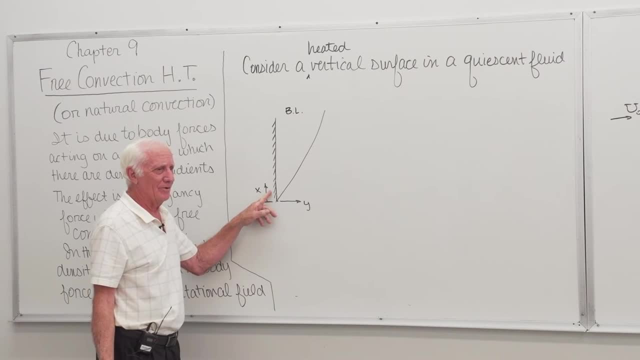 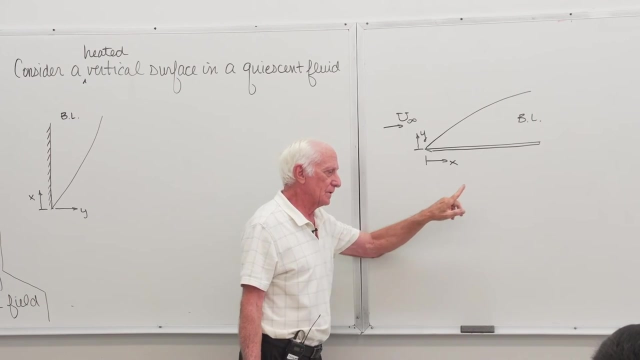 Why are you calling x in the y-direction? No, no, This is what it is. The x-direction is measured along the plate. Okay, The plate goes up. X goes up. X is measured along the plate. The plate's horizontal. X goes horizontal. 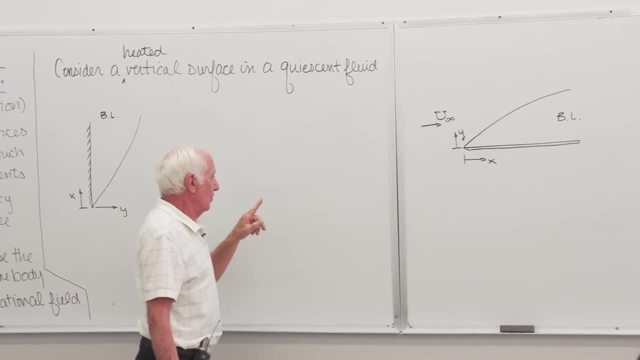 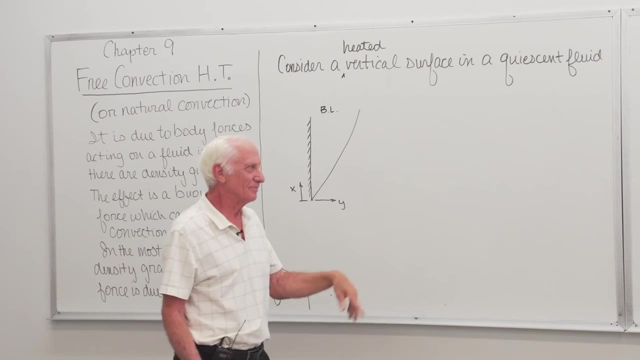 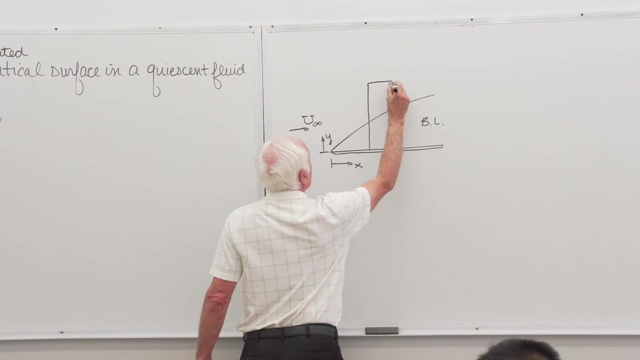 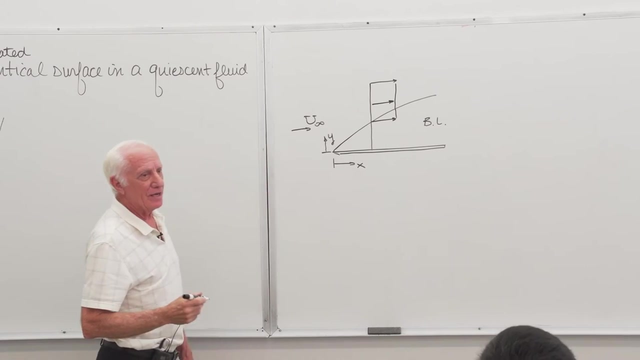 Y is measured normal to the plate up. Y is measured normal to the plate to the right. Okay, They're different, of course. All right, Look at what we had for the velocity boundary layer, officially called the hydrodynamic boundary layer. 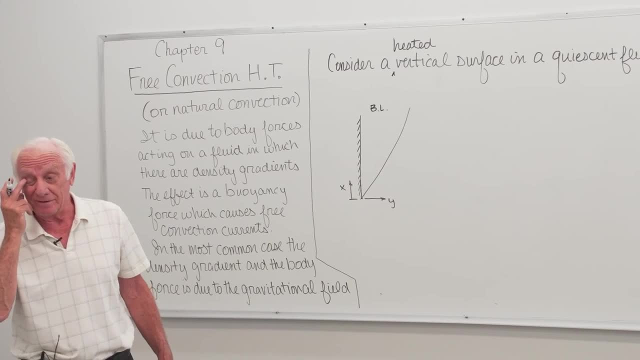 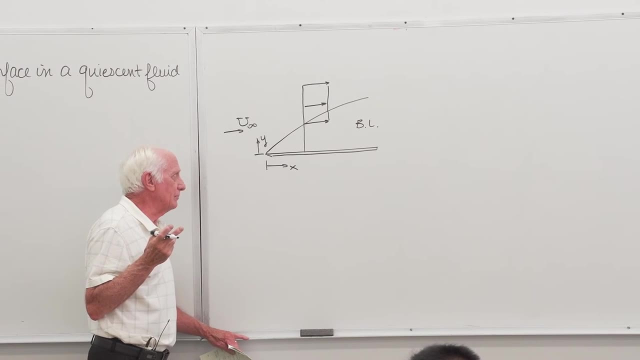 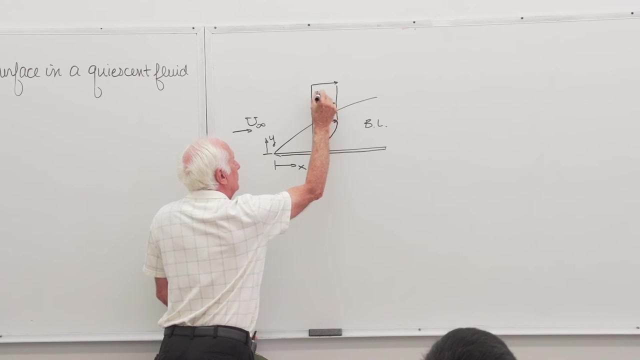 That's its official name. We use velocity boundary layer a lot. That's fine. Okay, Here's what's going on. No slip condition at y equals zero. Okay, What's the velocity at the plate? Zero, Zero, U, infinity u. okay. there it is. 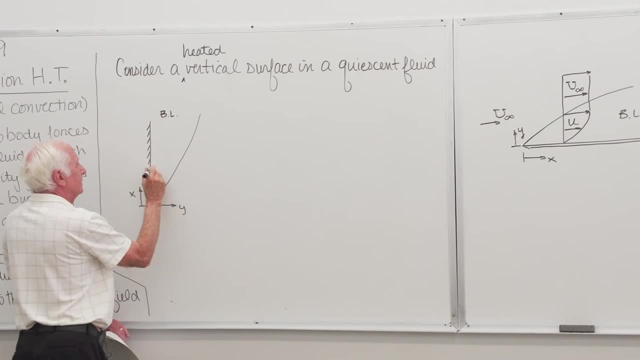 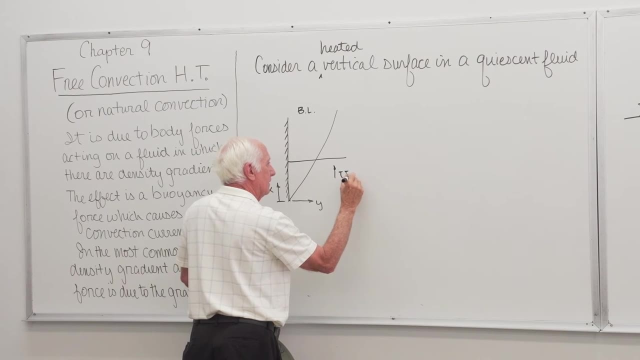 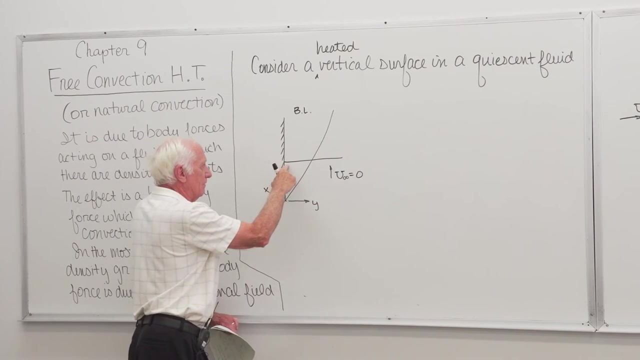 Let's draw the same thing for free convection. Oh, you got to be careful now, because you know what the velocity out here is. The velocity out here is zero. That's what the word quiescent means: zero. The velocity at the plate surface is zero. 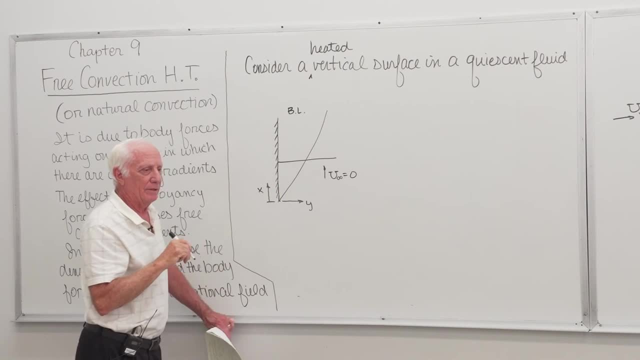 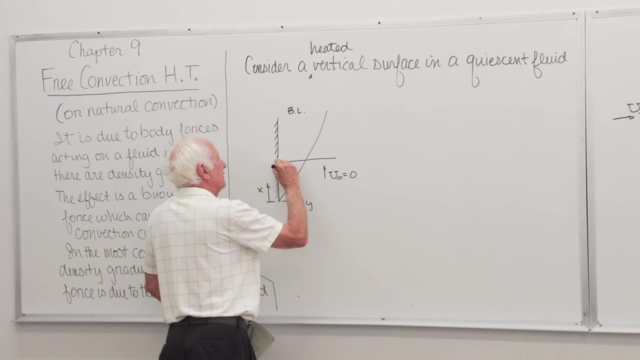 It's zero at the plate surface. It's zero at the edge of the boundary layer. It's zero at the edge of the boundary layer. Is it zero everywhere? Of course not. The fluid is rising. So now sketch this guy. So now here is the velocity. little u looks like that. 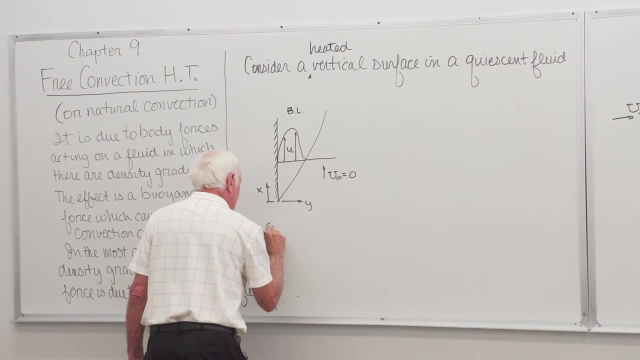 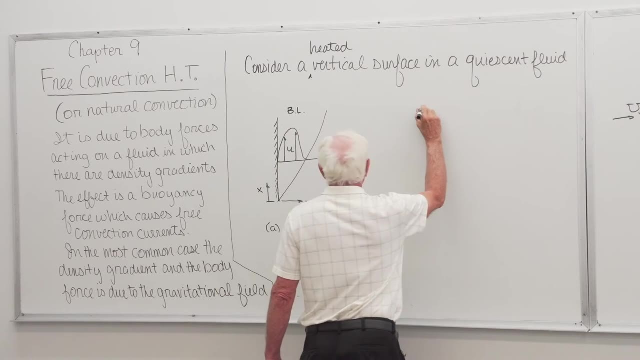 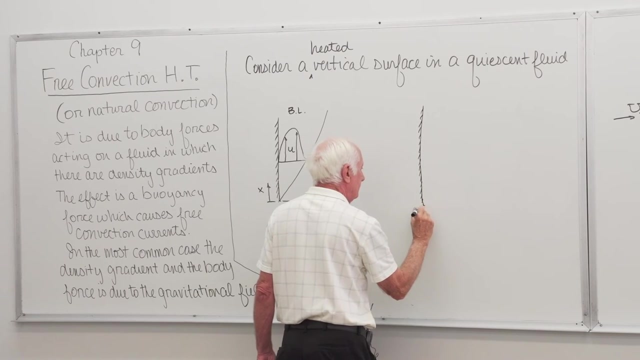 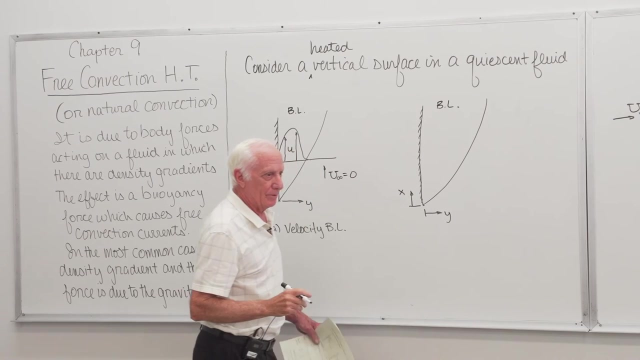 Okay, This is velocity boundary layer. Let's go back Now. we'll look at what's going on for the temperature boundary layer Again. we're measuring x along the plate. We're measuring y- normal to the plate. We get the temperature boundary layer. 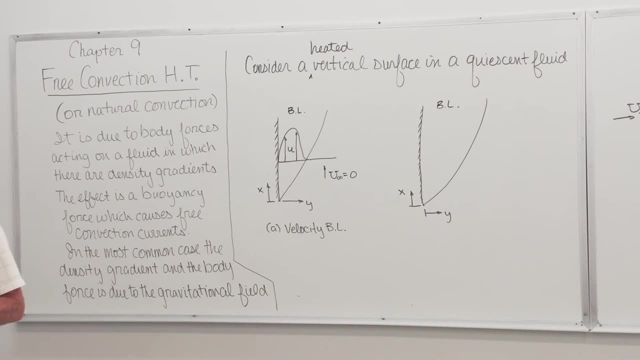 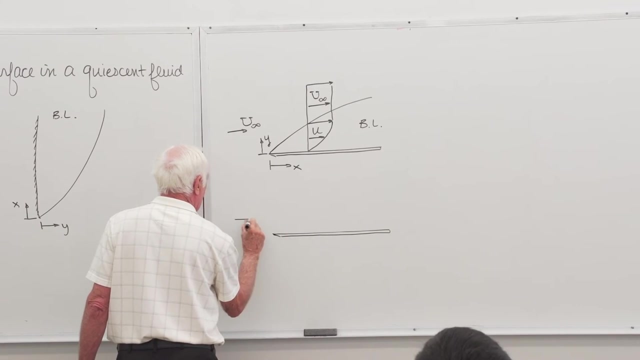 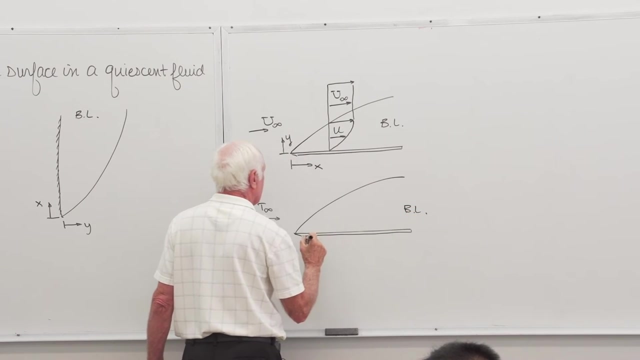 Officially called the thermal boundary layer, but we agreed on that term. But you know what? call it the temperature boundary layer. Let's go over here to this guy: Thermal boundary layer. Assume that the plate is heated. surface temperature of the. 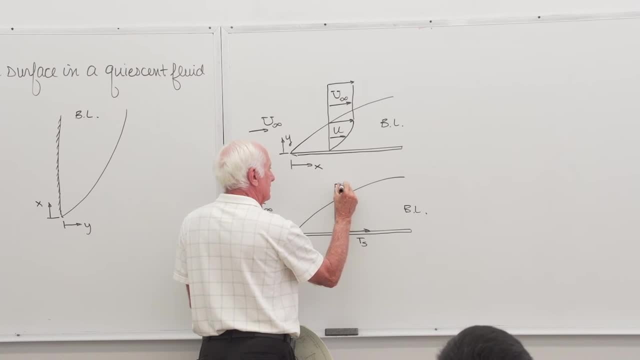 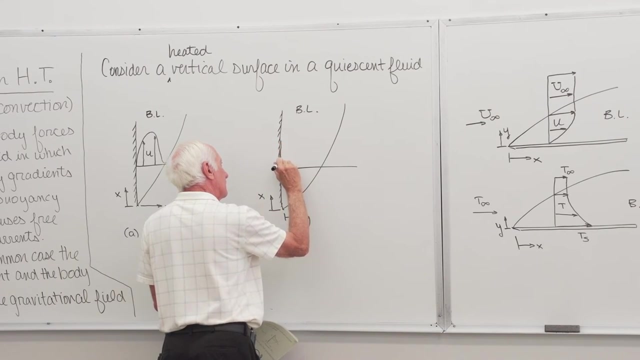 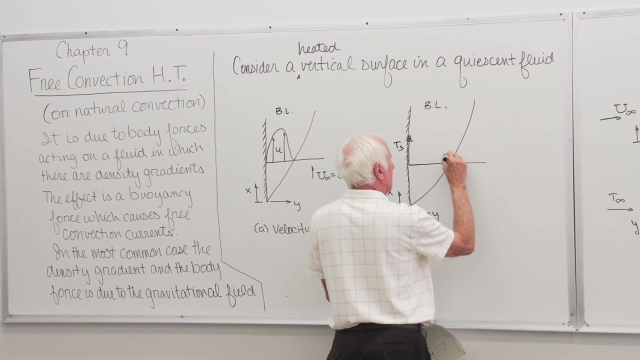 plate TS. Assume the free stream velocity temperature is lower. Draw the thermal boundary layer There it is Over here. draw the thermal boundary layer. Assume the surface is heated and assume that the temperature of the free stream is less than that. 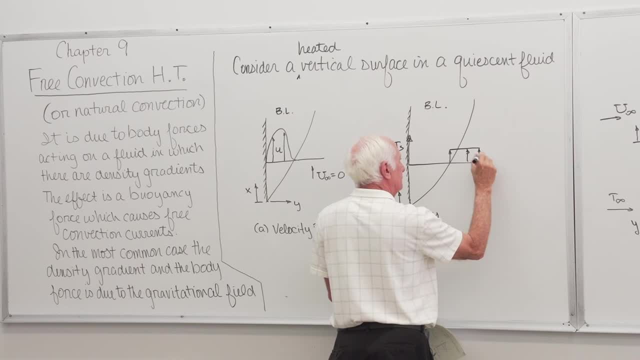 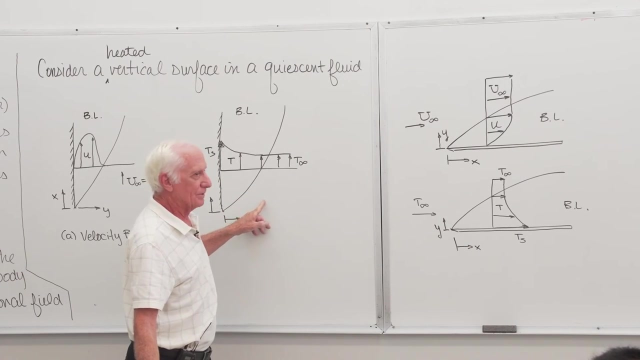 So it looks like that. So the temperature boundary layers look very similar for chapter 7, chapter 9, but the velocity boundary layers look really different. Okay, this is B, the thermal boundary layer, temperature boundary layer. Okay, so that's what we're dealing with. That's for a. 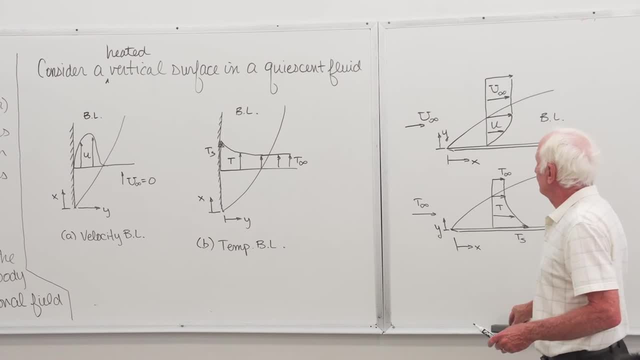 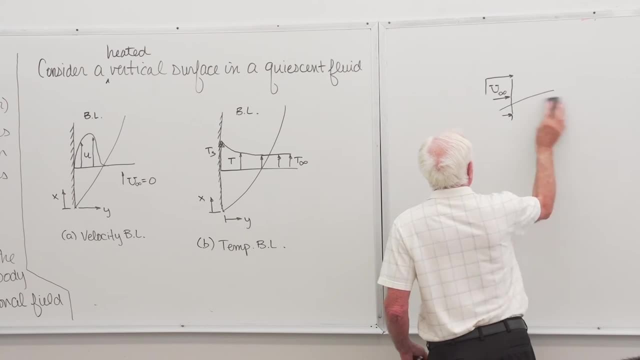 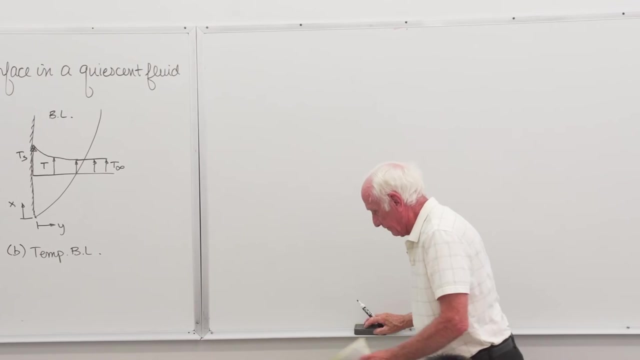 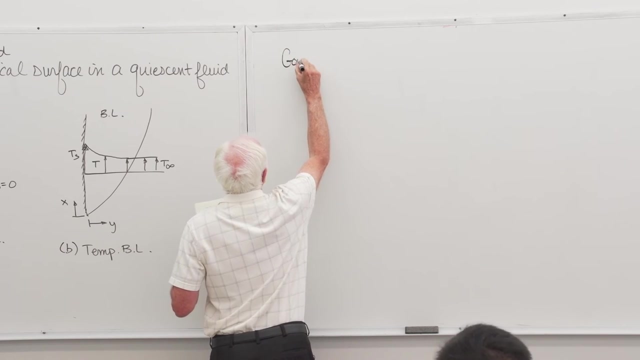 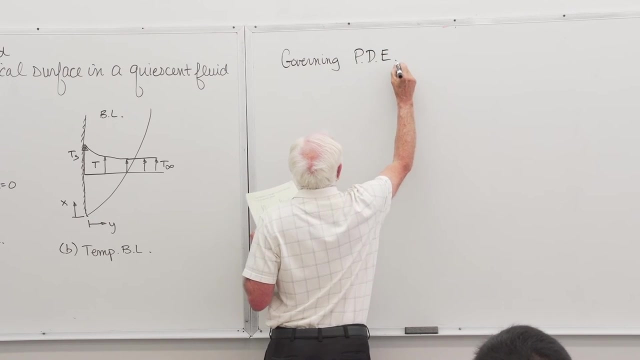 vertical plate: heated vertical plate. Okay, so now we going to, with that understanding, we write down the governing partial differential equations. So what we're going to write now, governing PDEs, And start off with continuity conservation of mass. This is a different. 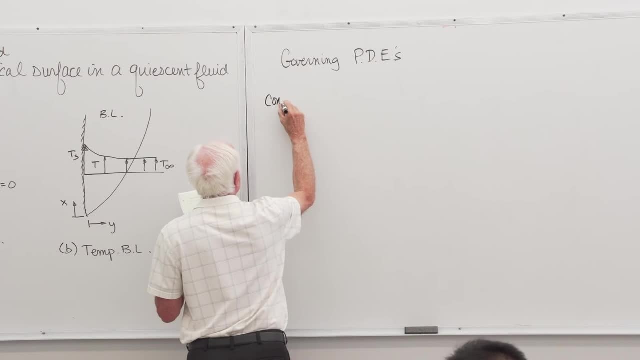 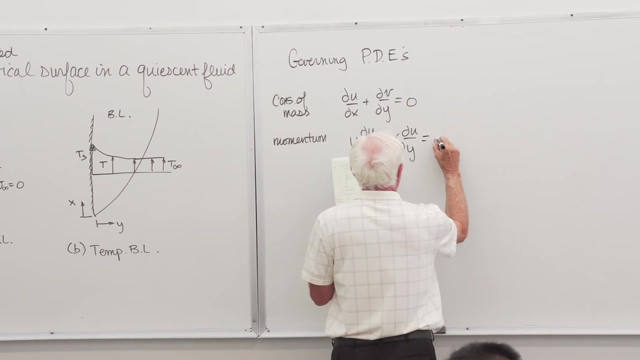 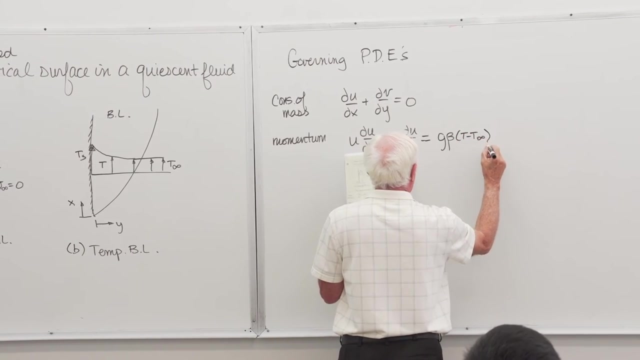 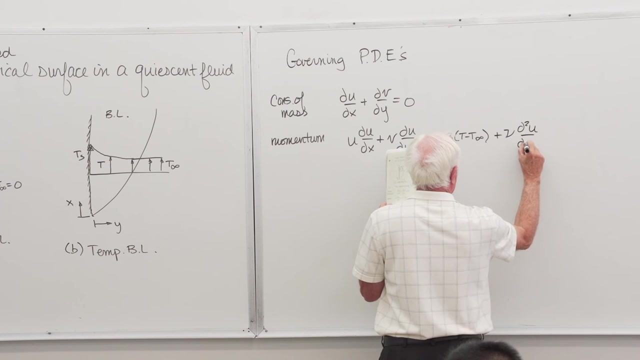 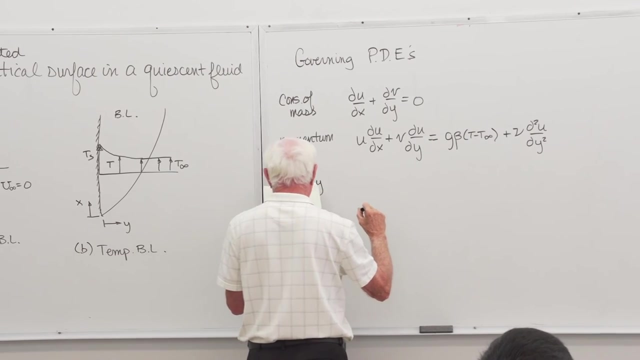 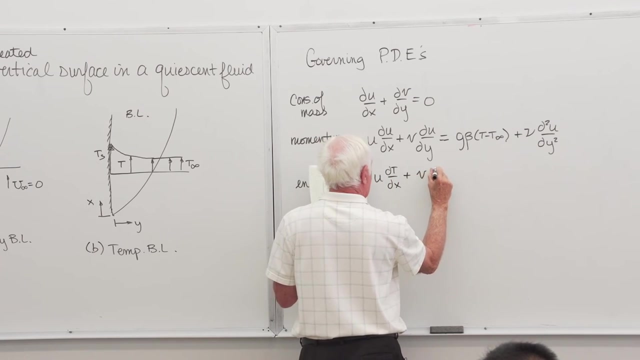 period of time. And what we're going to do again is we're going to write down the governing partial differential equations. So what we're going to do is we're going Go to momentum equation. Finally, of course, energy. All right, 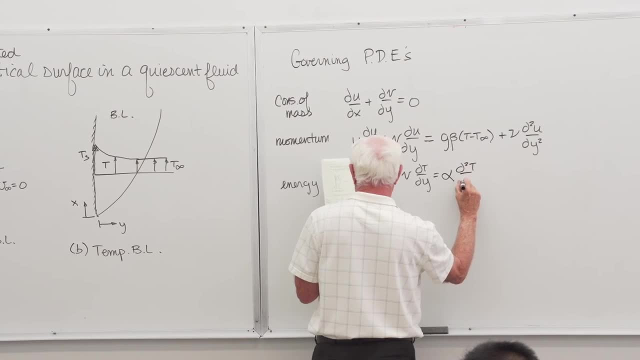 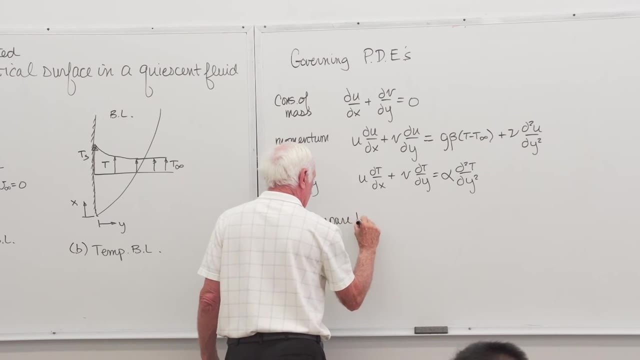 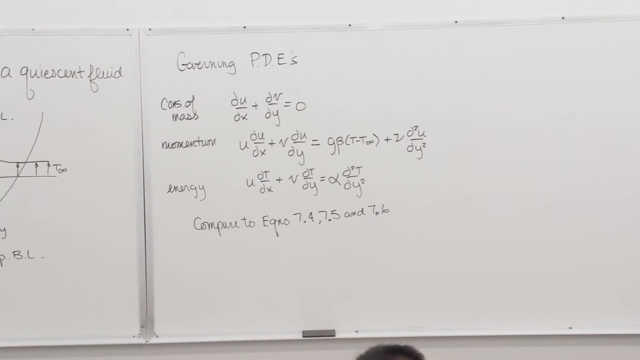 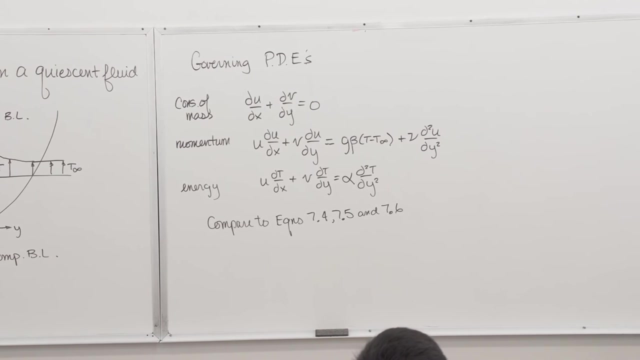 So we need to take a look at some more. So we need to take a look at some more. We set this problem up in Chapter 7, and we wrote down in Chapter 7 the same three equations: conservation of mass momentum and energy. 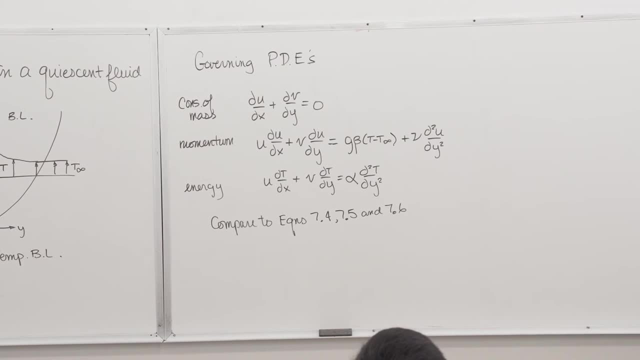 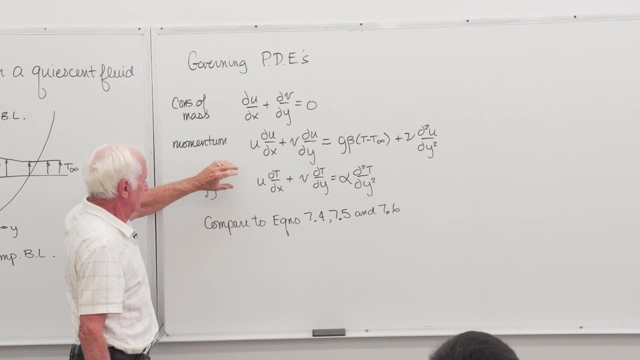 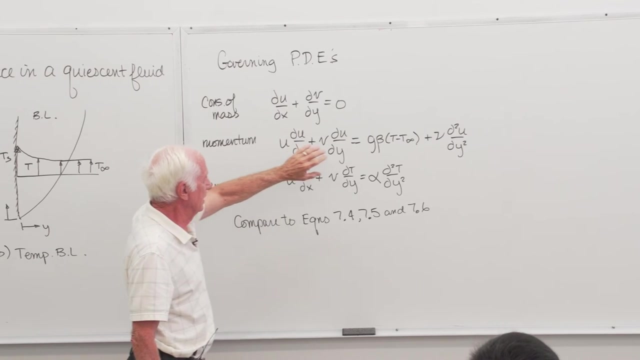 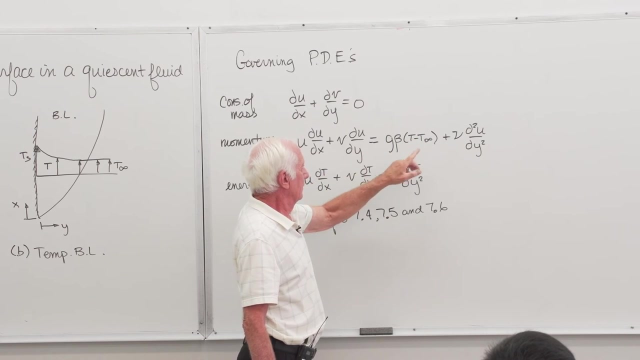 They're almost identical, but they're different. They're different because, well, conservation of mass was identical, conservation of energy, or energy, was identical, But the x momentum here is different. What's different? This term wasn't here. This term is due to the buoyancy effect. 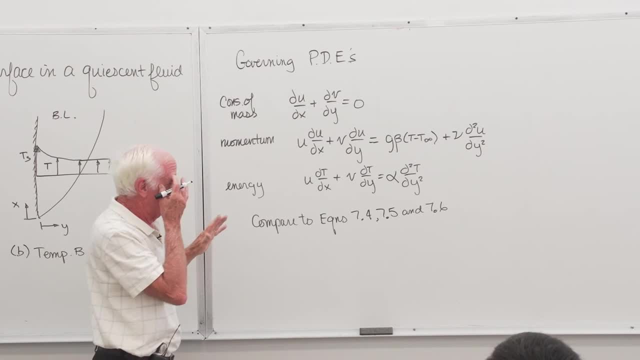 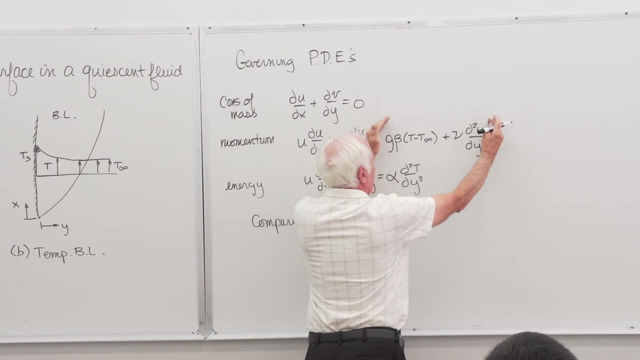 That's the buoyancy force. So you know what momentum is. This side equation is: the change in momentum is equal to the forces acting on. What's this force? It's got viscosity. This is a viscous force. What's this force? 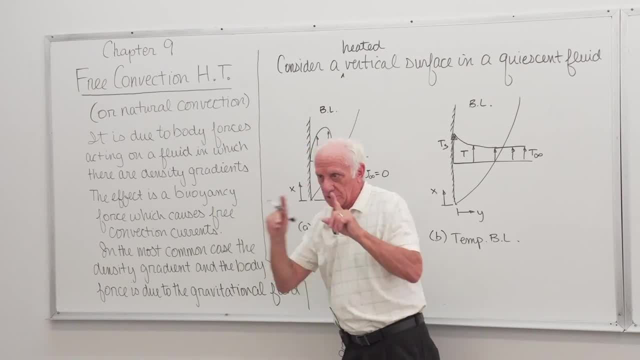 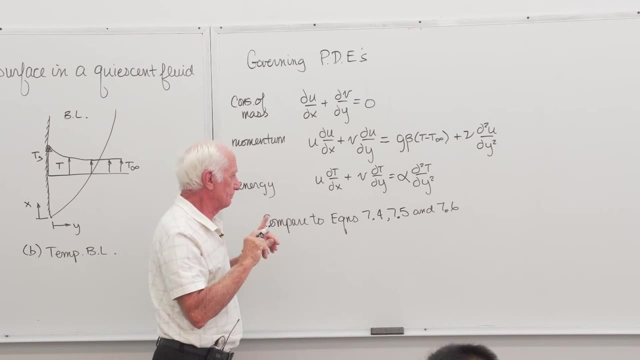 This is the buoyancy force. two forces, Viscous force, buoyancy force. So that's the difference. This is called the buoyancy force, But it complicates matters because previously- in Chapter 7, we could uncouple these equations and solve. 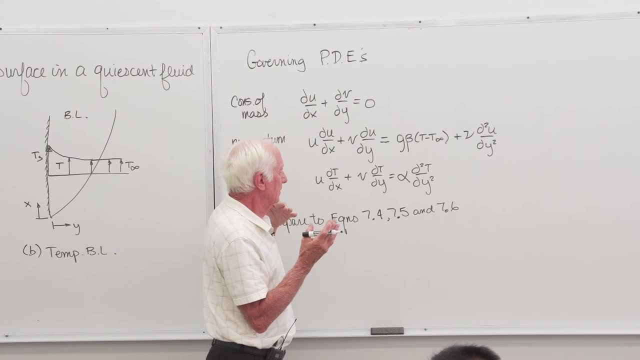 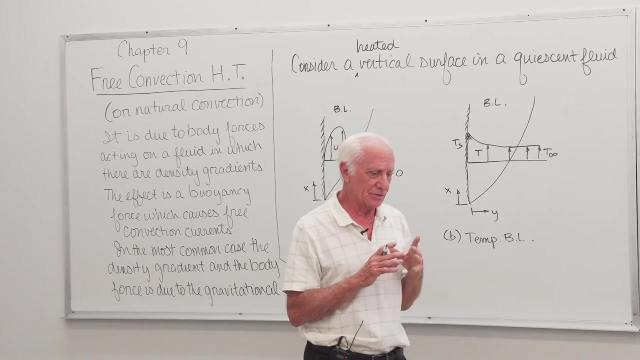 them each one separately, for instance. Now the problem is I see temperature in momentum and I see temperature in energy, and that makes it a lot more difficult. They're called coupled equations, So to solve these are much more difficult because the equations are coupled. 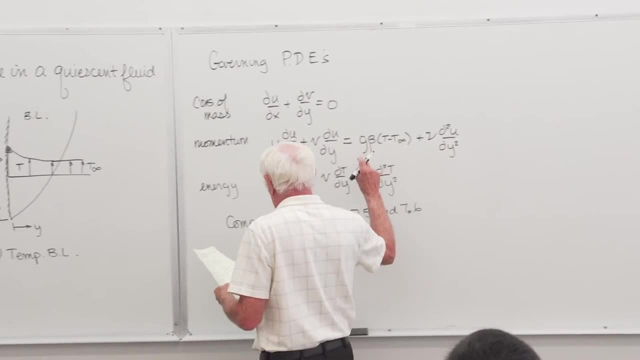 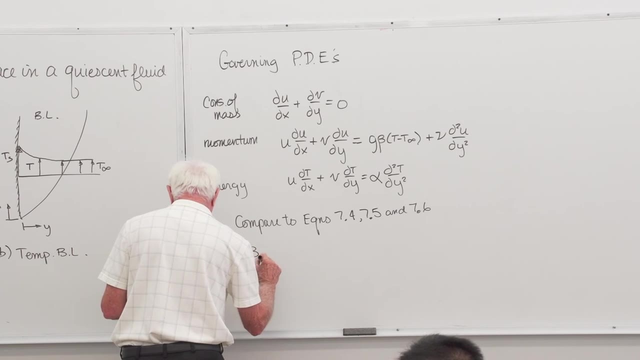 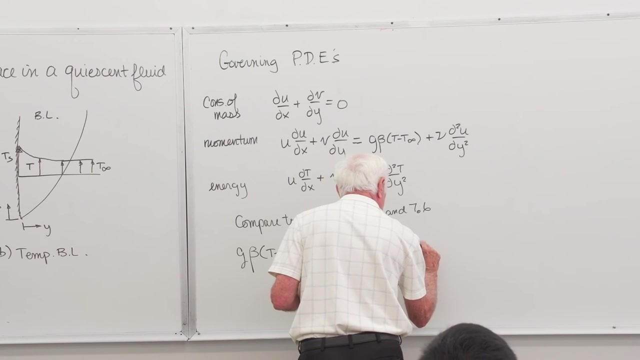 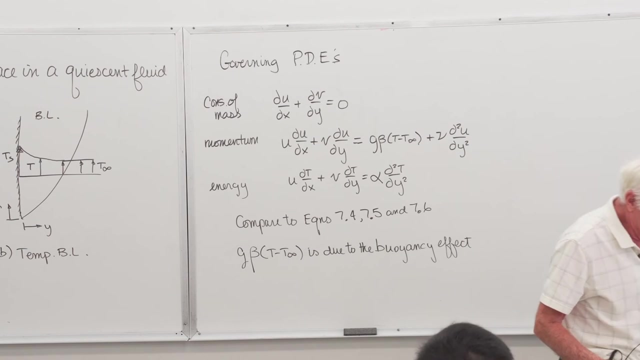 Okay, Let's mention what this guy here is: G, Beta, t minus t. infinity is due to the buoyancy effect And I'll put: let's see, I think I'll put that up here. Okay, You know what G is: gravitational constant. 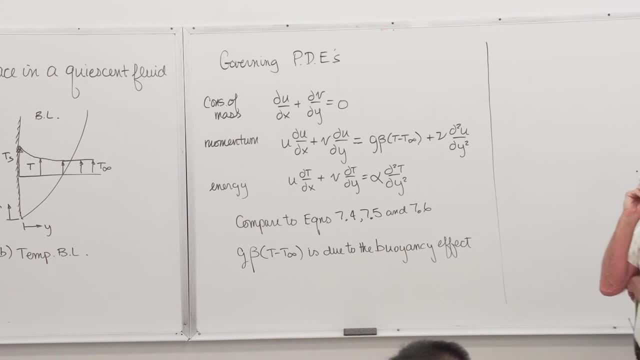 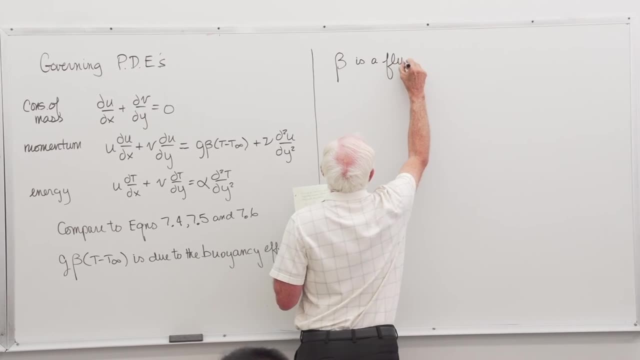 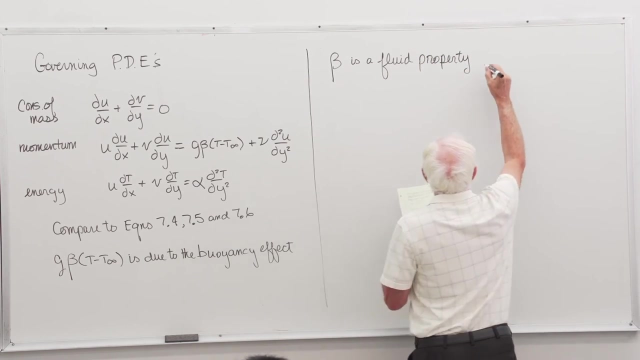 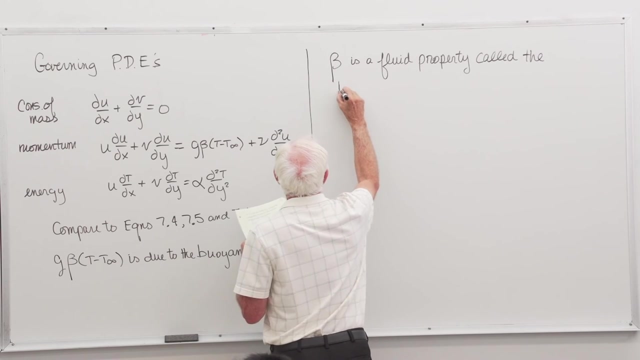 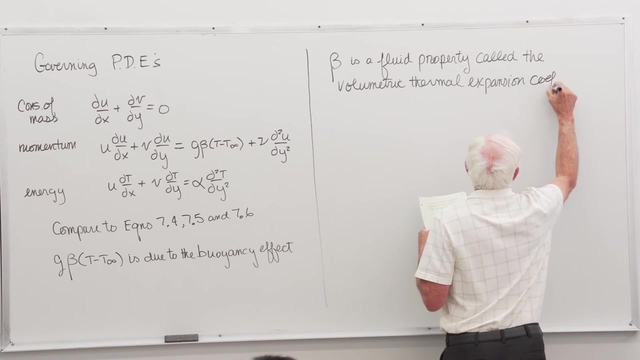 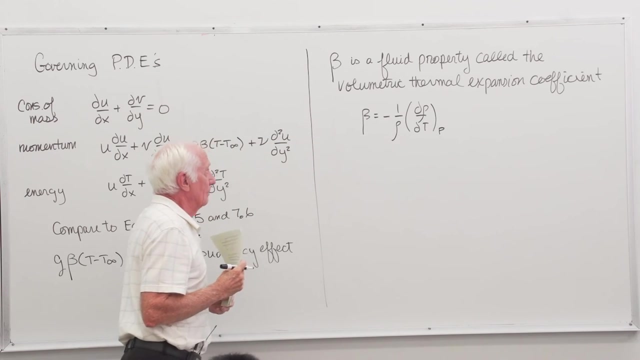 We'll use 9.81.. Beta- Beta is the new thing, So Beta is a fluid property. We'll call the volumetric thermal expansion coefficient Thermal. it was defined like this: Beta minus one over density times the partial density with 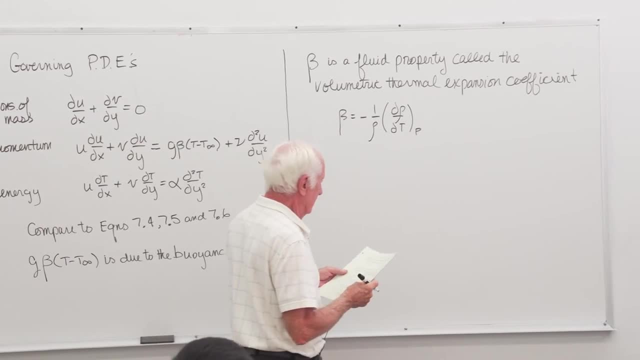 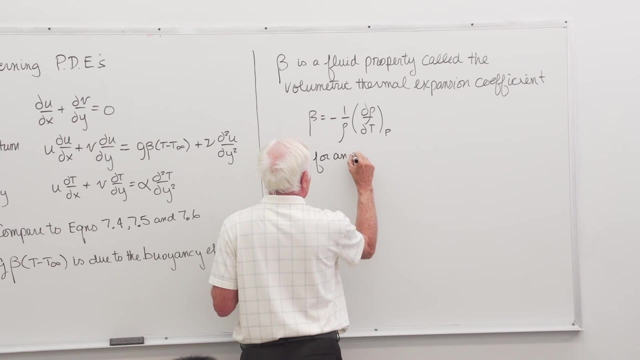 reflected temperature, holding the pressure constant. And if you use an ideal gas, beta is one over the absolute temperature. So beta is at least one over density. That's what I call a vector Okay, And that's what the temperature is. So beta minus 10 to the power of 2 is the temperature. 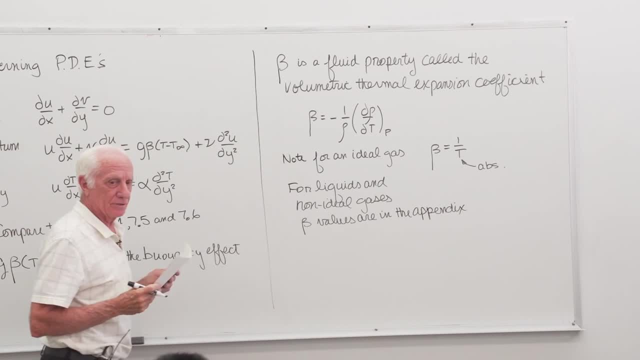 And then I'll draw a line here And I'll go back in and I'll say: okay, so I wrote down my orange in the middle And then I'll write down the temperature. And then I'll write down the temperature if it's not an ideal gas or liquids. 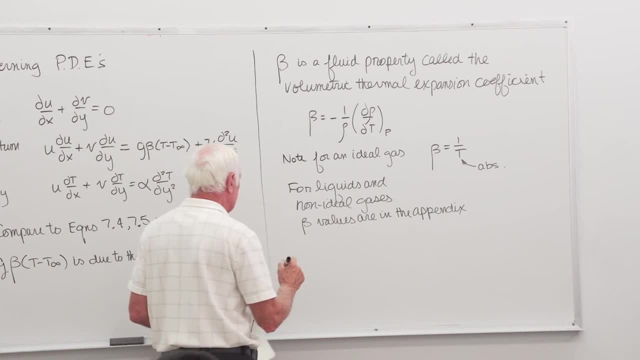 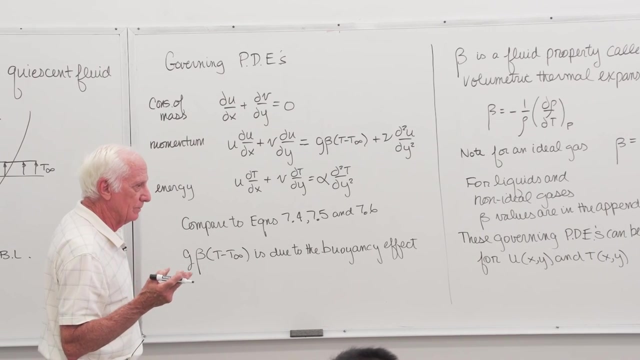 the beta values are given there. Now the equations can be solved. The results give you the velocity at any point x and y in the velocity boundary layer or the temperature at any point x and y in the temperature boundary layer, But they're not given in equation form. 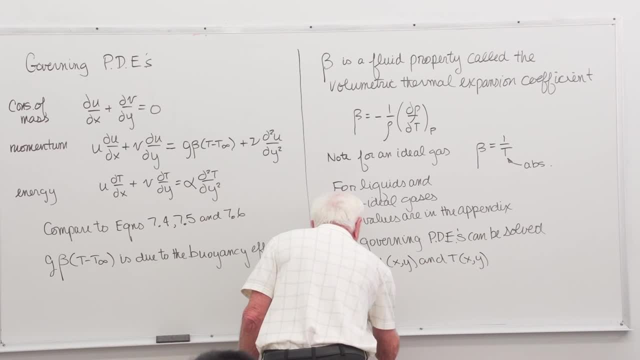 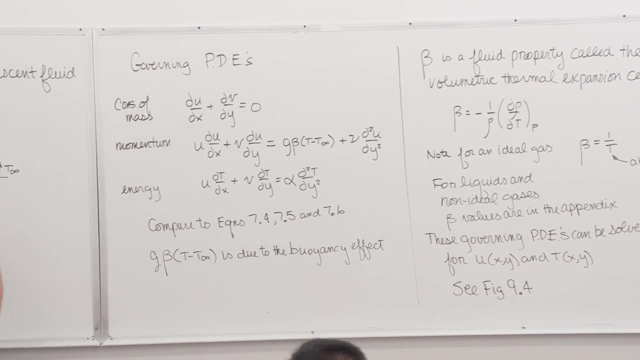 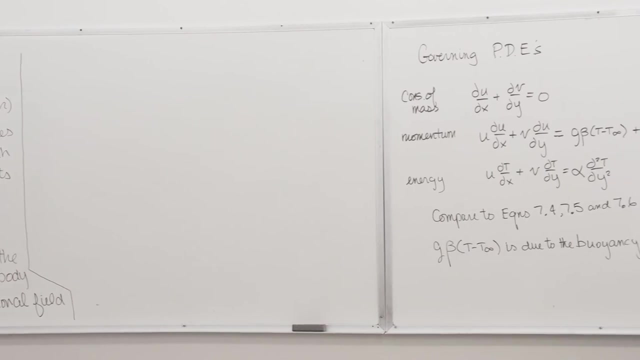 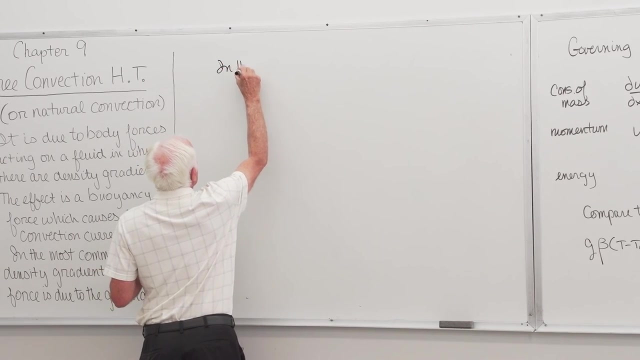 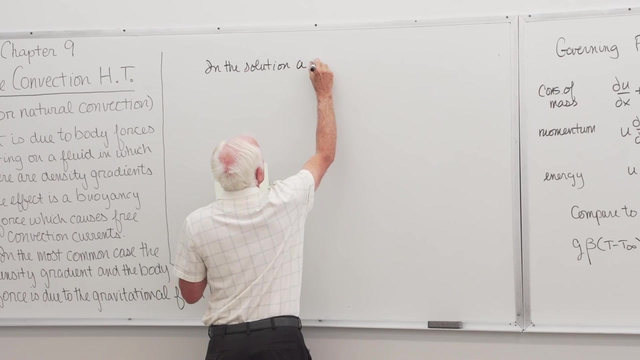 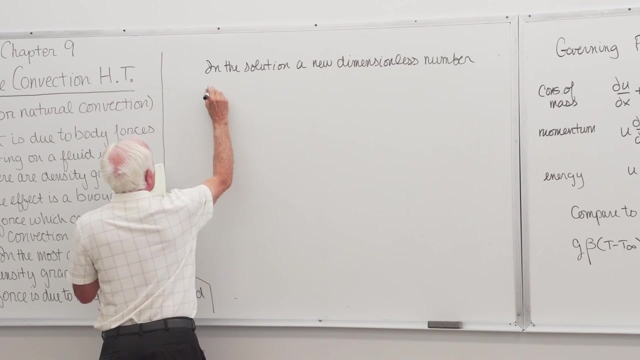 they're given in figure 9.4.. That figure gives both the velocity and the temperature. In the solution a new dimensionless number is defined as g R as a function of L g, Beta temperature difference, Ts minus T. infinity L cubed divided by Nu squared. 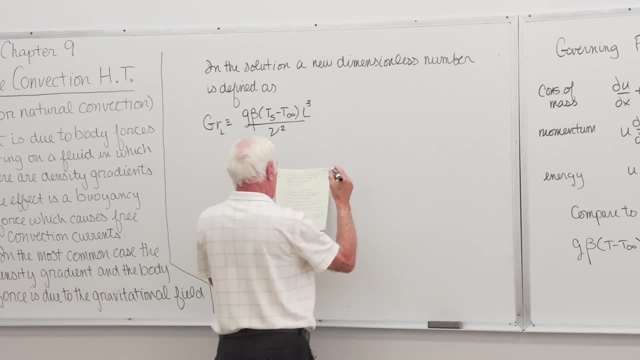 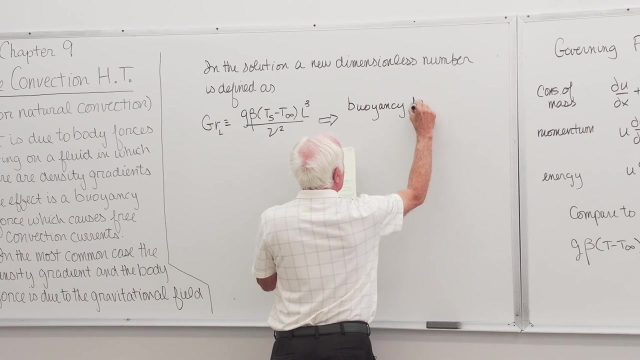 It's dimensionless. It can be interpreted like you did. but it's dimensionless, It can be interpreted like you did. and it can be interpreted like you did in fluid mechanics in terms of a ratio of forces: the buoyancy force divided by 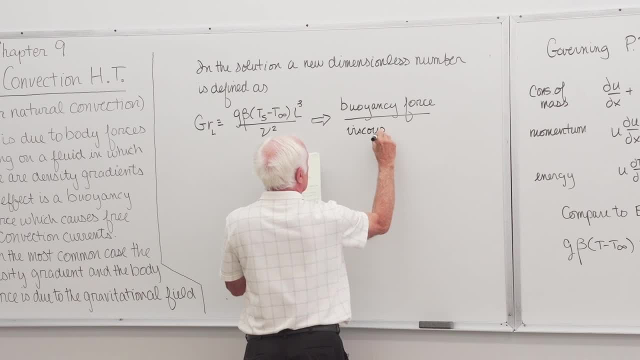 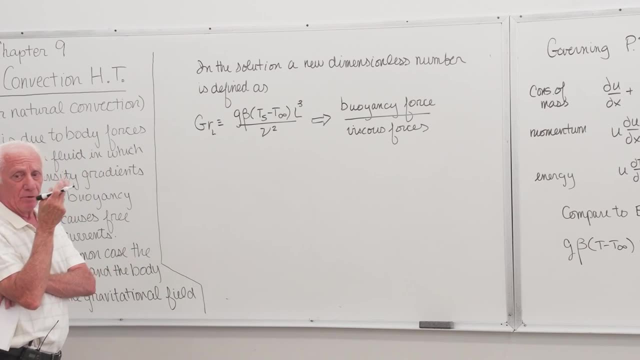 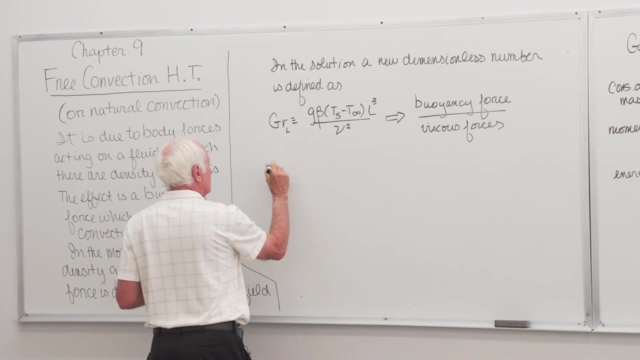 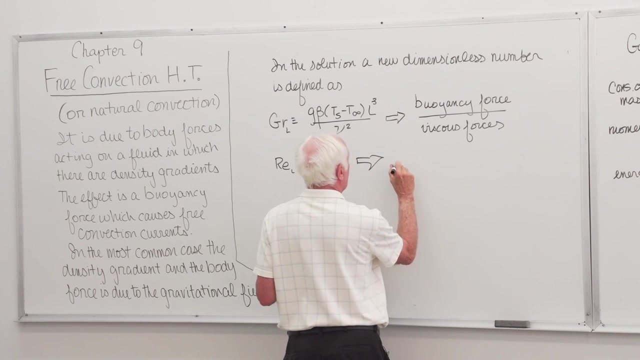 the viscous forces. So the Grashof number is related to the buoyancy effect, the buoyancy force. If you go back to fluid mechanics and relate that as a ratio of forces, the Reynolds number U, infinity, L over nu, that can be interpreted as a ratio of forces In 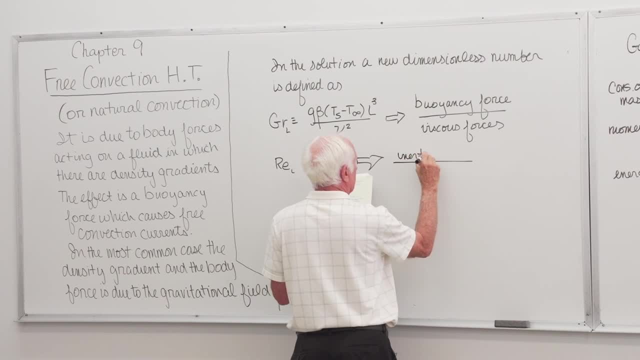 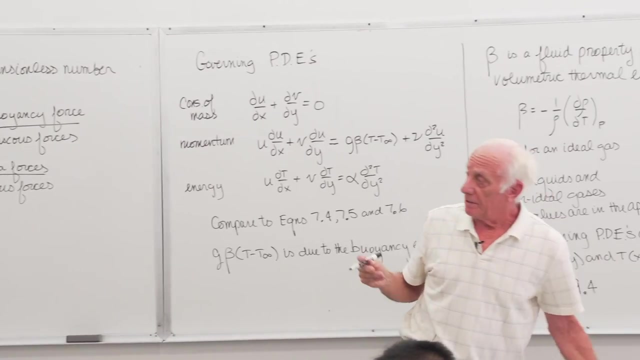 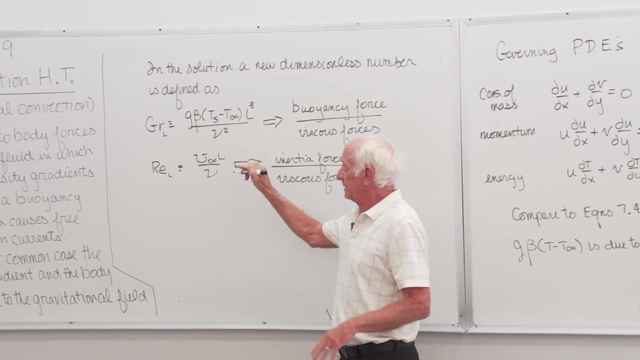 this case it's the inertia forces divided by the viscous forces. So in chapter 9,, free convection, of course, the buoyancy force is really, really important. That's what created the motion. So in chapter 9, this is an important dimensionless parameter.